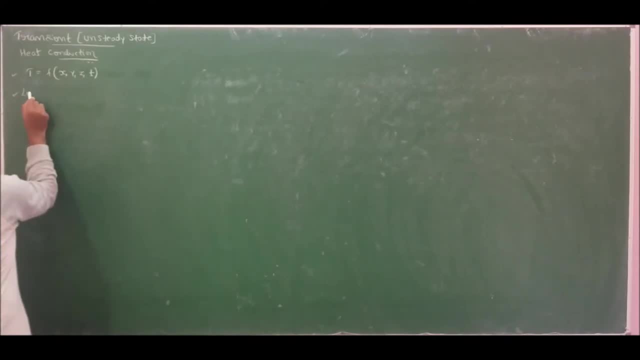 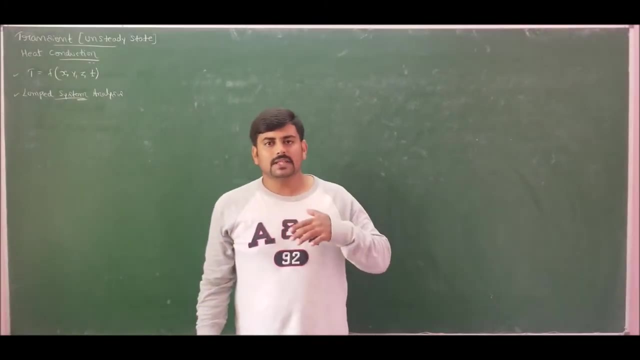 heat transfer for our temperature. please visit amtrakfullskillscom Lumpur. system analysis is nothing but an assumption in which temperature is a function of time alone and it does not vary with respect to space and coming for lumpur system analysis. a better understanding will be, for an example, if I consider an slab and heat transfer through. 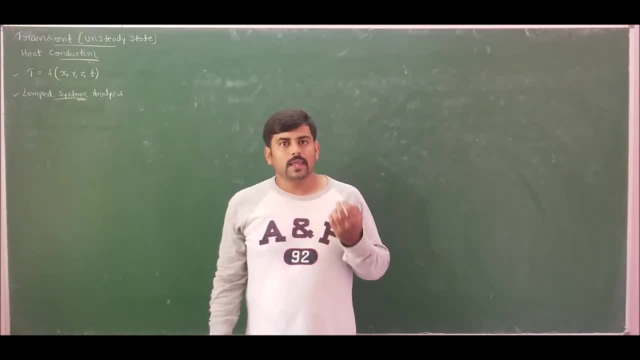 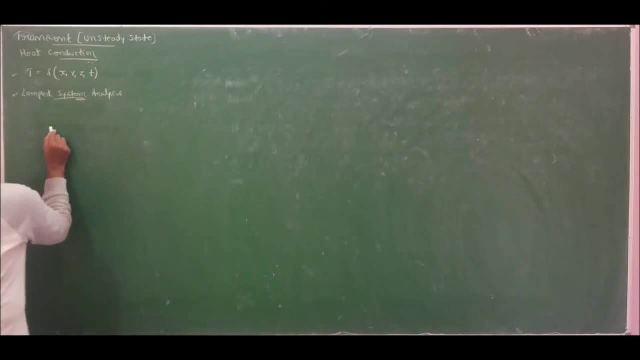 slab by both conduction as well as convection. the conduction resistance is already known to us. the conduction resistance for a slab is given by L, by Ka, which is nothing but conductive resistance, whereas the convective resistance is given by 1 by He. these two people already. 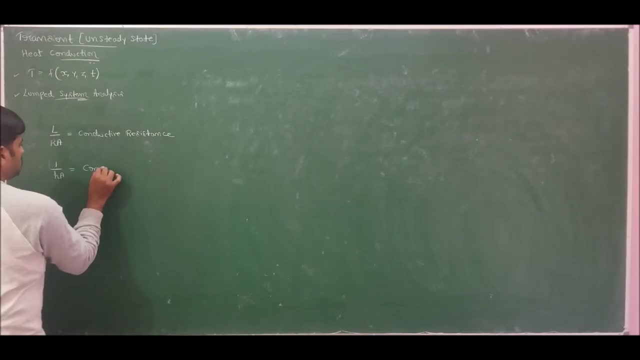 know during our discussion on module 1. now, if the conductive resistance is very, very small compared to convective resistance, then R conduction is very, very small compared to R convection. then we can neglect the variation of temperature which we have already demonstrated. so now we will discuss about a slag and heat. 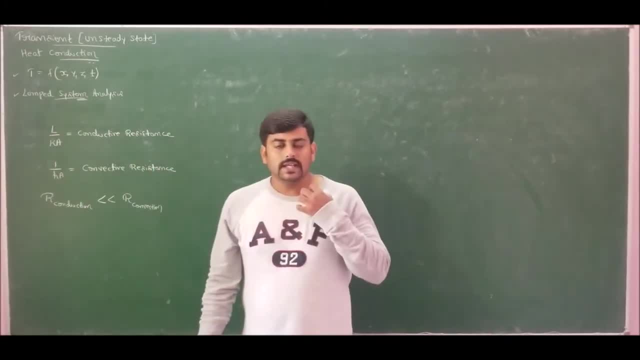 transfer the system and we can consider that the entire system is of same temperature when the conductive resistance is very less compared to external convective resistance. so if i take this condition into account, then temperature is a function of only time and it is independent of space. so 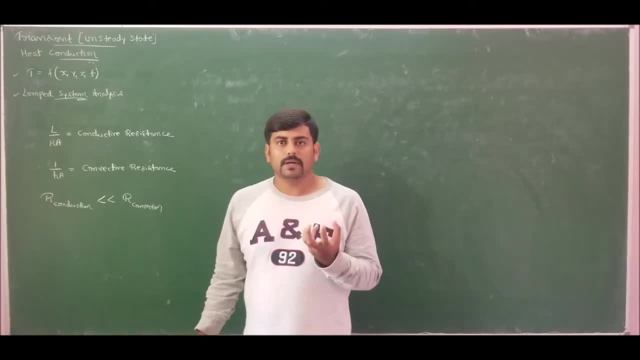 overall system can be considered as an one lump, hence the name lumped system analysis. so in case of lumped system analysis, temperature is a function of time alone. so over the space temperature won't change within the system. the entire system will be at a same temperature. so 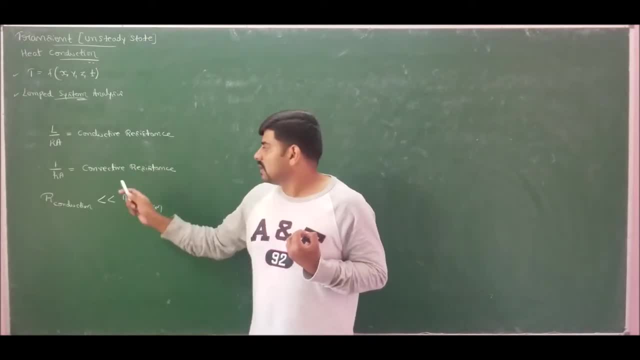 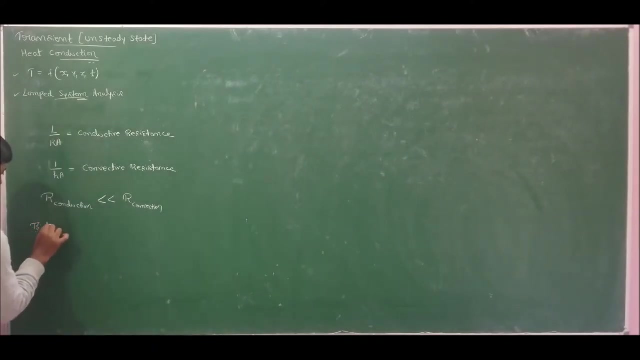 this holds good if the conductive resistance is very small compared to external convective resistance. so the ratio of these two, conductive resistance to convective resistance, is termed as biot number. so biot number plays a major role in conducting lumped system analysis. so the ratio of these two is nothing but biot number, which is specified as: resistance due to conduction by resistance due to external convection. for lumped system analysis to be valid, the conductive resistance should be less than convective resistance. so therefore, for lumped system analysis, biot number should be very, very less than one. so therefore the sufficient condition to apply. 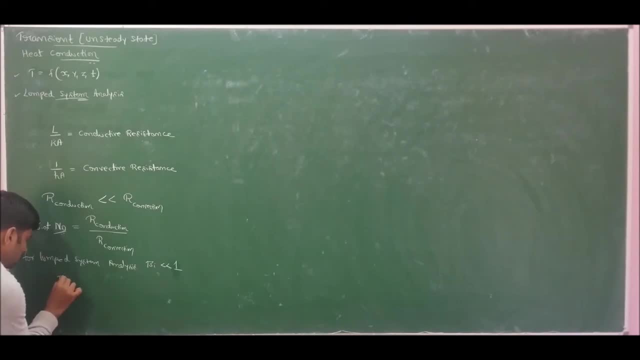 lumped system analysis is that the biot number is less than 0.1 is enough to conduct lumped system analysis. so therefore, if i substitute these two in the equation of biot number, i can define the biot number as hlc by k. so this is the formula for biot number. so i will derive this equation of biot number. 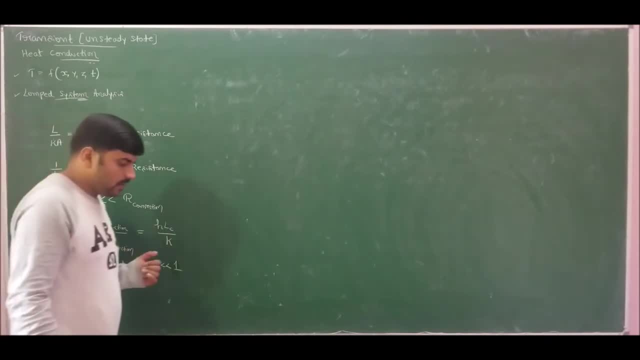 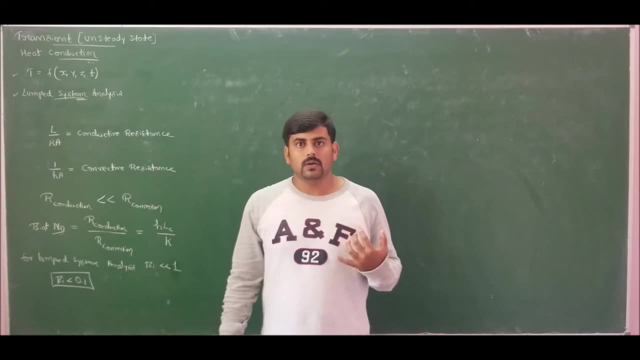 right now. so hope you understood what is the meaning of lumped system analysis. lumped system analysis is an assumption in which the temperature is a function of time alone and it is independent of space. so this holds good if the internal conductive resistance of a system is very. 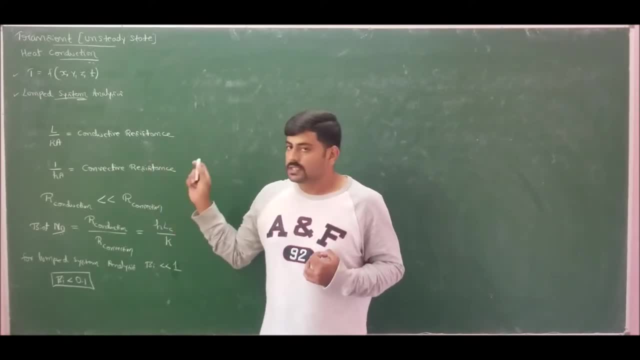 is very less compared to external convective resistance. so during that situations the entire system can be considered to be as a one lump and the entire system will be at an same temperature at any point on the system. if you measure, the temperature remains same. the temperature varies only with respect to time. 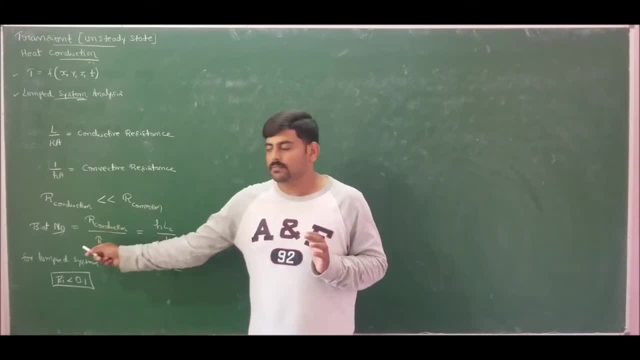 so if i take the ratio of these two, we'll get a dimensionless number called biot number. so biot number plays a major role in determining, in analyzing the lumped systems. so, as i As I discussed, the Bayard number should be very, very less than 1 to apply lumped system. 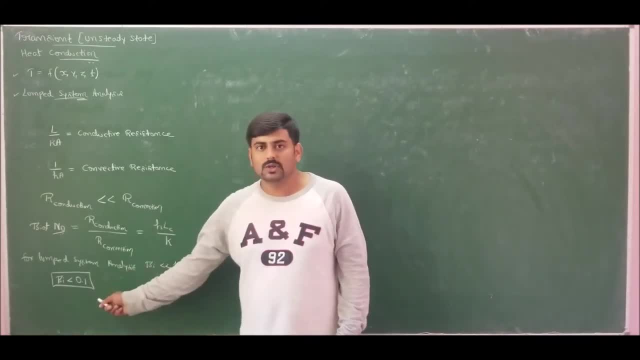 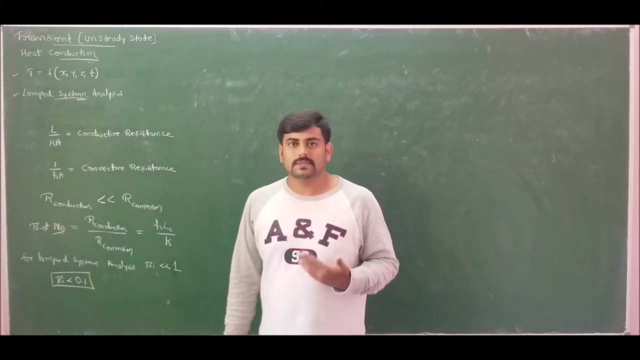 analysis. The sufficient condition is that if Bayard number is less than 0.1, we can go for lumped system analysis. Hope you understood. Now let us derive an expression for temperature distribution in one dimension- transient heat conduction- and also let us derive expressions for cumulative heat transfer and total heat. 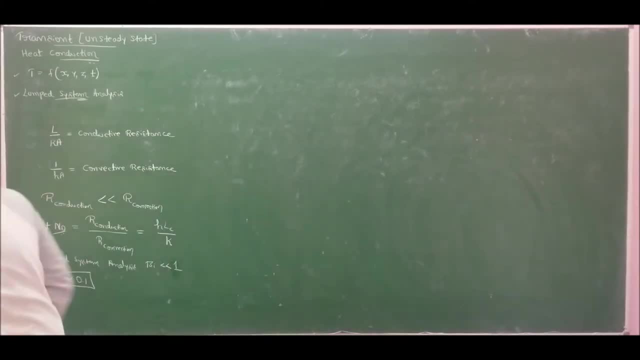 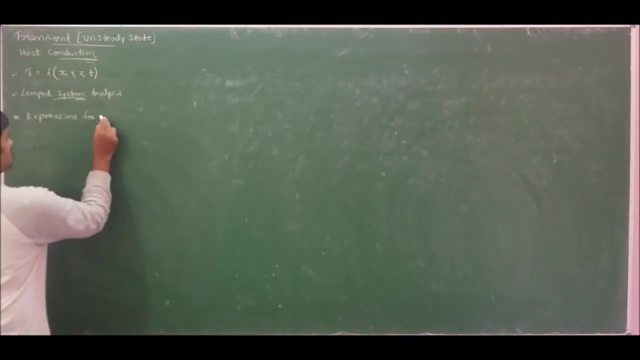 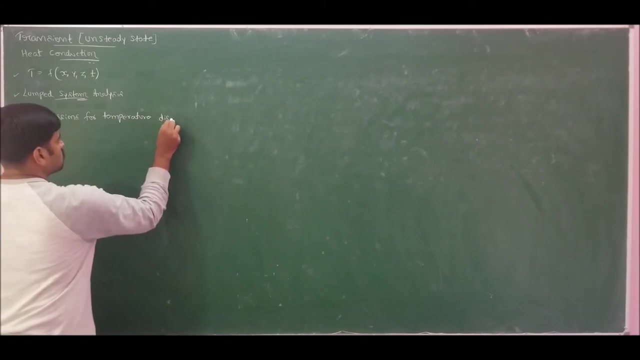 transfer. That is, we are ready to derive expressions for temperature distribution. Wait, We are ready to derive expressions for cumulative heat transfer, instantaneous heat transfer and cumulative heat transfer. Now let us consider a hot sphere. Let me consider a hot sphere. 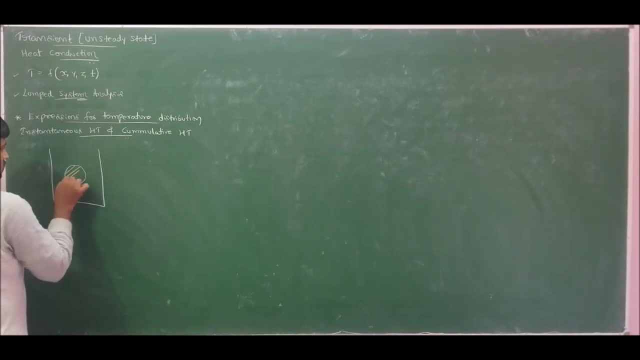 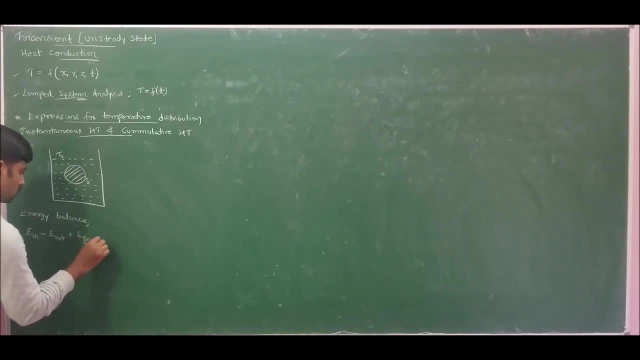 generated must be equal to change in internal energy of the control volume. So energy in minus energy out plus energy generated must be equal to change in internal energy of the control volume. So now we are not supplying any energy to the system, So therefore energy in is zero. 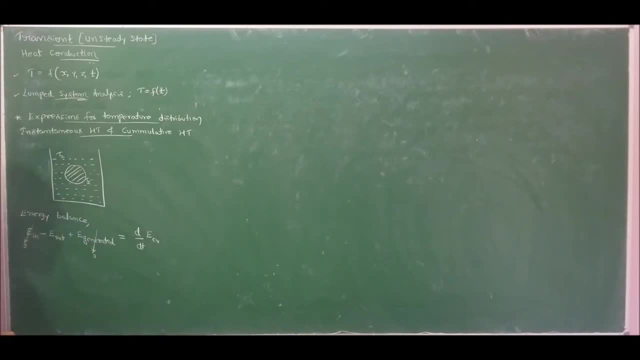 There is no any energy generation, So energy generation is also equal to zero. So therefore energy moving out is because of convective heat transfer. So therefore we know that the formula for convective heat transfer is given by HCA surface. 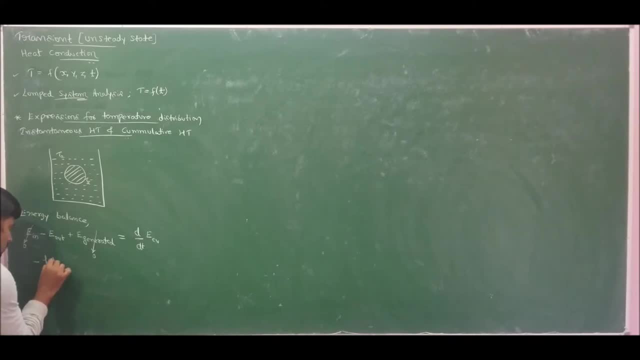 times T minus T, infinity. Let us consider the temperature of the surface as T, And this is. I am neglecting the radiation heat transfer. I am taking only the heat transfer only because of convective mode, And this must be equal to changing internal energy of the control volume. 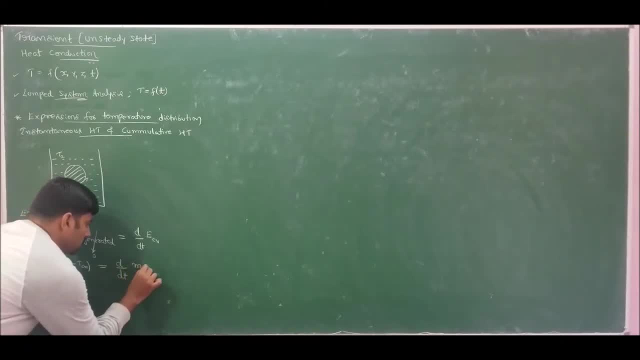 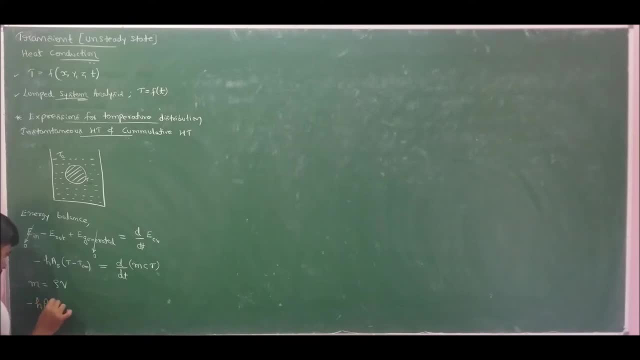 If I substitute and solve, I will get minus HAS T minus T. infinity is equal to d by dt of rho Vc T. So let me use capital T for temperature. Now, as I said, for transient heat conduction I am going to use T minus T. 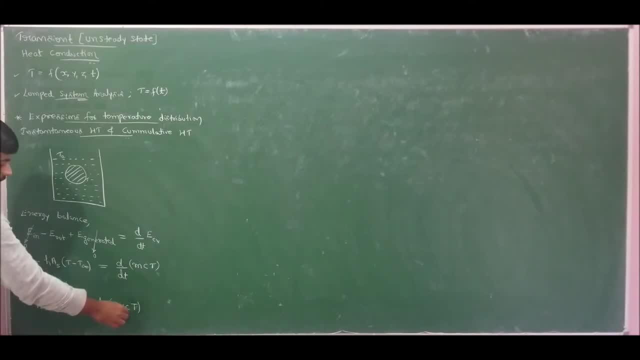 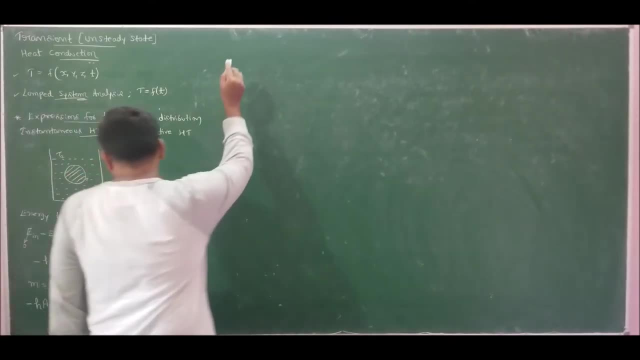 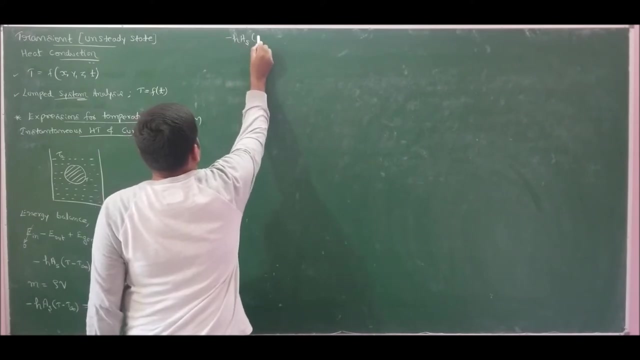 So let me use capital T for temperature. Now, as I said, for transient heat conduction, temperature is not constant with respect to time, because temperature varies with respect to time. So therefore, if I differentiate the right hand side and formulate, I will get minus, HAS T, minus T infinity. 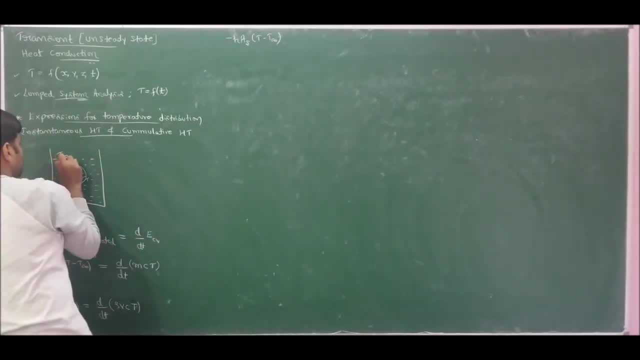 Here the ambient is T infinity. Do not get confused. T A is in the right hand side, T I is in T, but T infinity I am considering. So this must be equal to rho Vc by dt. so this must be equal to rho Vc by dt. 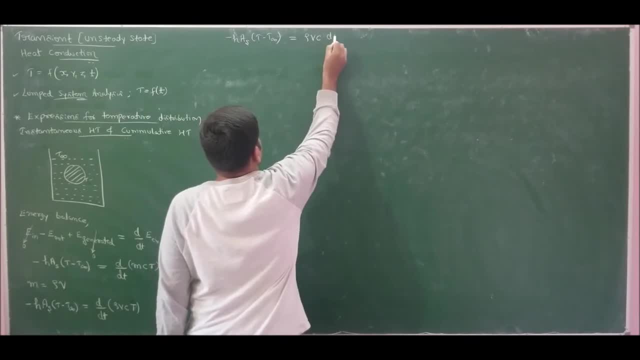 t A is in the right hand side, So this must be equal to rho Vc by dt. t A is in the left hand side, So this must be equal to rho Vc by dt. So this must be equal to rho Vc by dt. 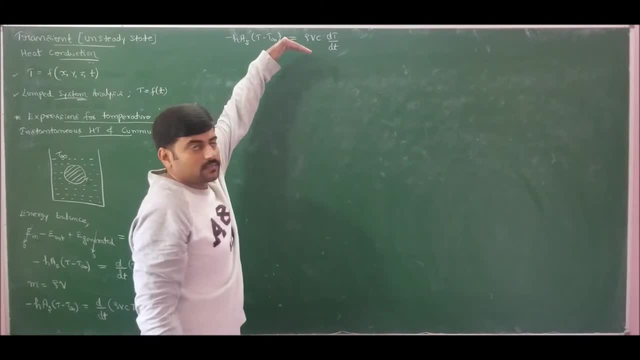 capital T stands for surface temperature. capital T stands for surface temperature, T A is in the right hand side. S S is for time, S R stands for time. Now, if I rearrange the terms, I will get minus HAS by rho Vc into dt is equal to 2.. 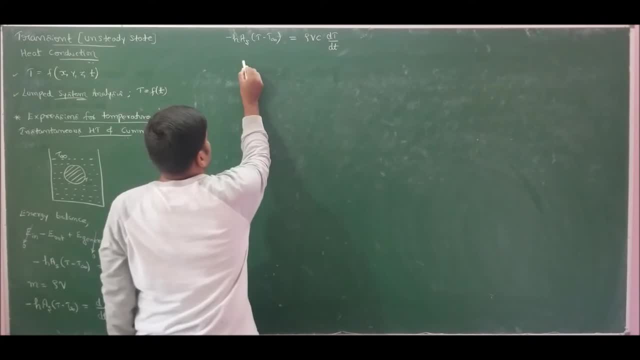 So I would write Stein or Stein Z would be square root less than value minus H AC into 1 group. Now if I rearrange the terms, I will get minus h i s by rho v c into d t is equal to 1 by t minus t, infinity times d t. 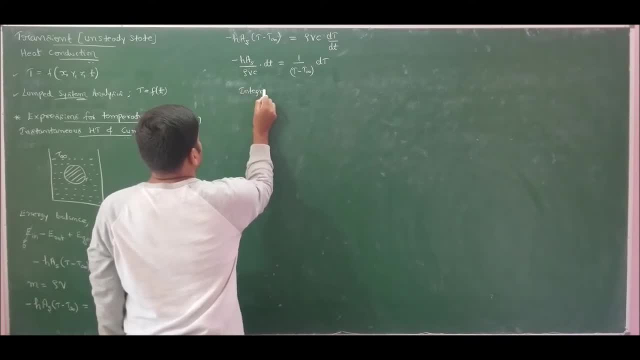 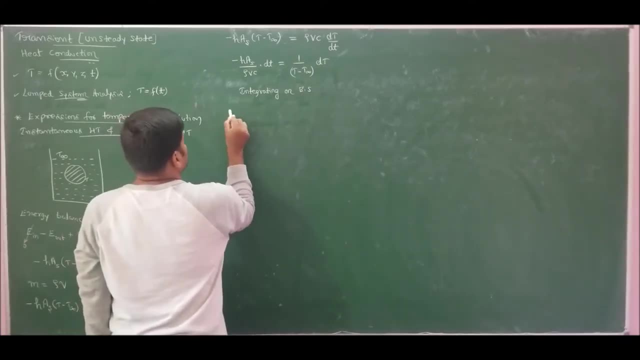 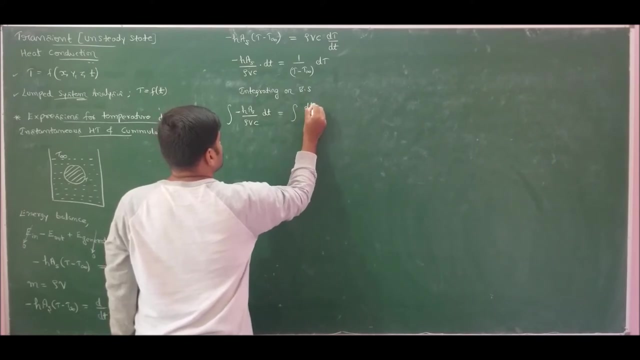 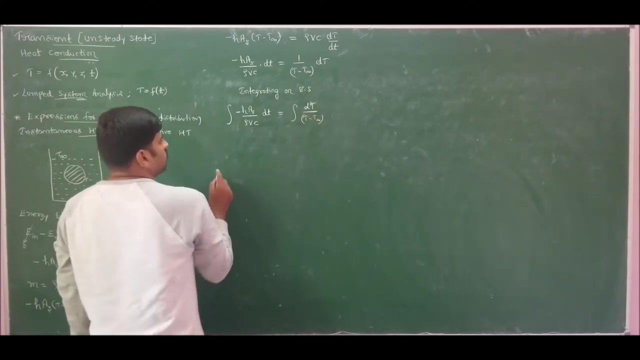 So integrating on both sides. if I integrate both sides, we have integral of minus h i s by rho v c d t is equal to integral of d t. temperature minus t, minus t, infinity times d t. So if I conduct integration, since it is indefinite integral, I will have constant of integration also. 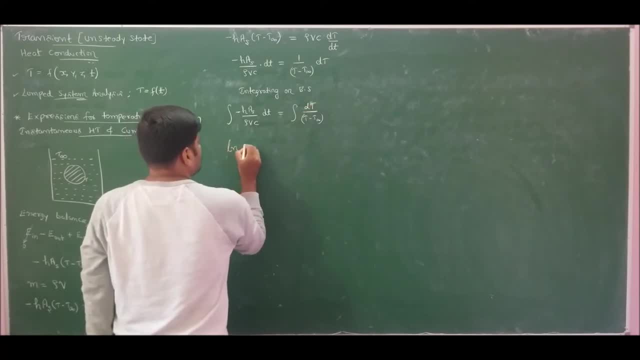 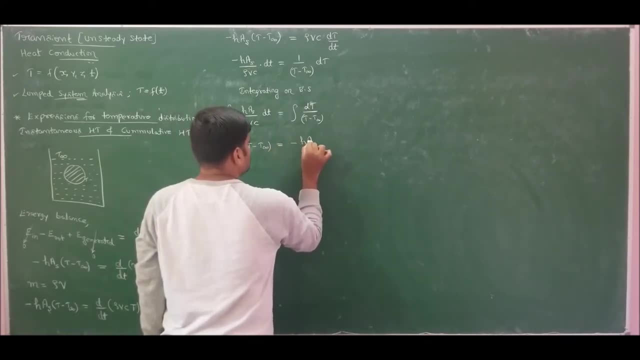 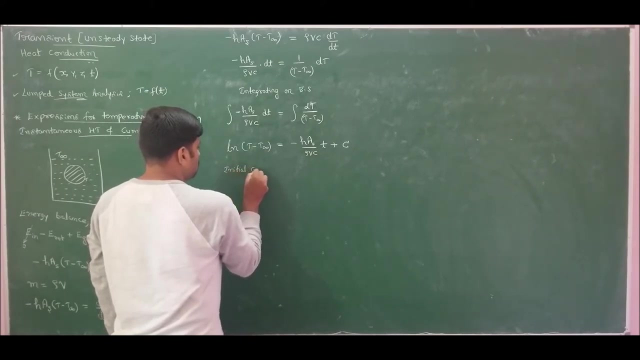 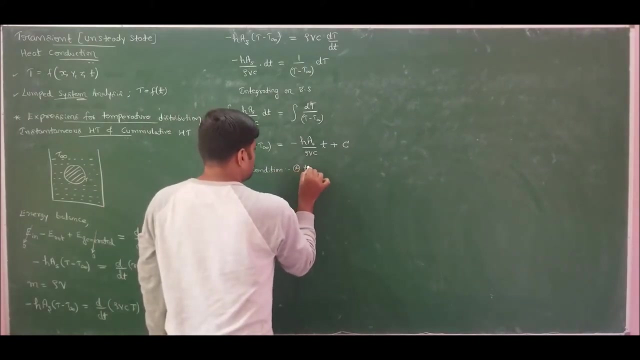 So integral of 1 by x is log x. So therefore it is log of t minus t. infinity is equal to minus h i, s by rho v, c times plus constant of integration c. Now we have initial condition. The initial condition is that at time t is equal to 0, the temperature of the surface is t. initial 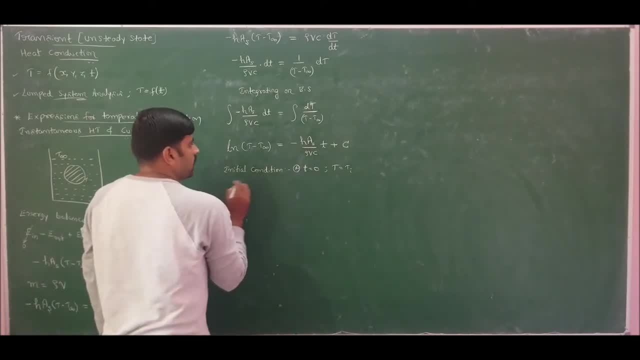 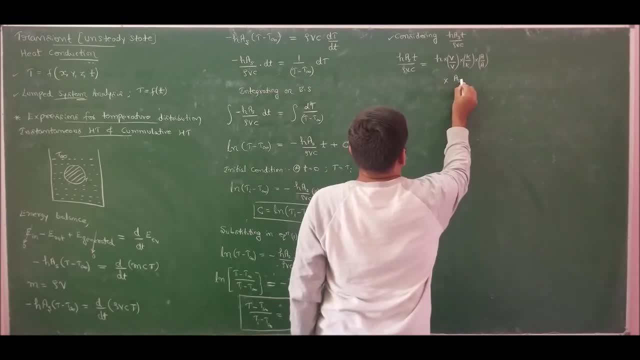 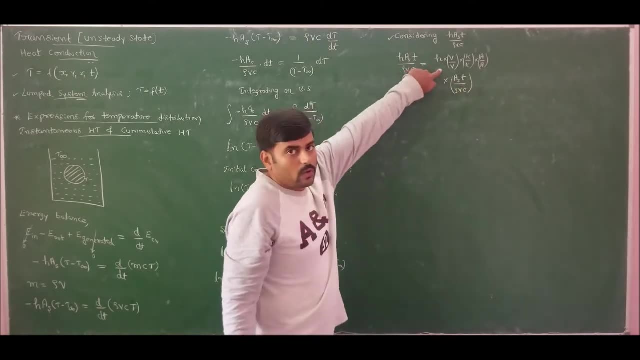 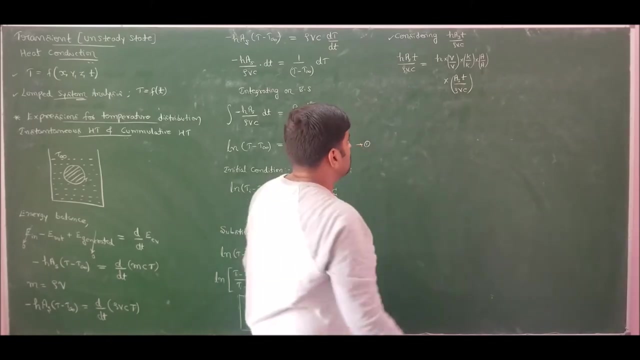 And then keep other terms as it is, As t by rho v, c. So I multiplied and divided by volume, multiplied and divided by thermal conductivity, K multiplied and divided by area A, multiplied and divided by area A. So now, if a rearrange this: 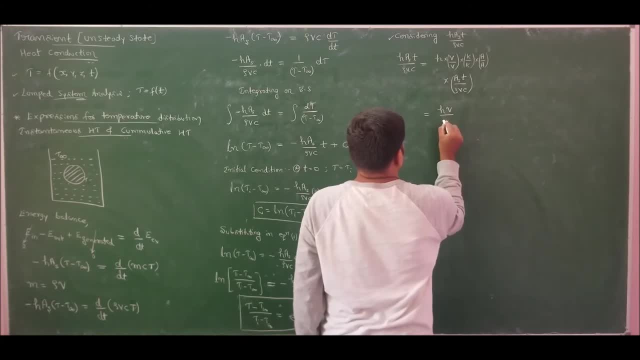 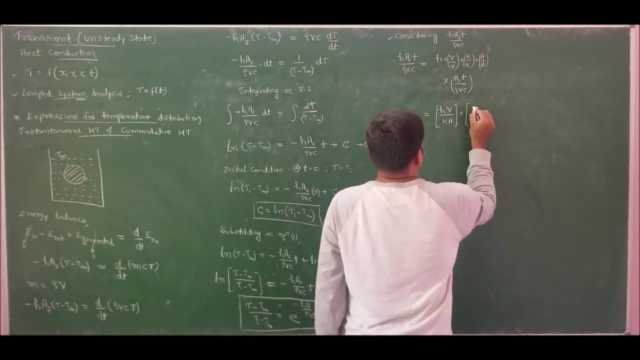 I can write this as Hv by Ka As one term. I will take Hv by val C As one term. I will take Hv by val C by K a into. I can write this as we have 88 a square T divided by B square, Rosie. 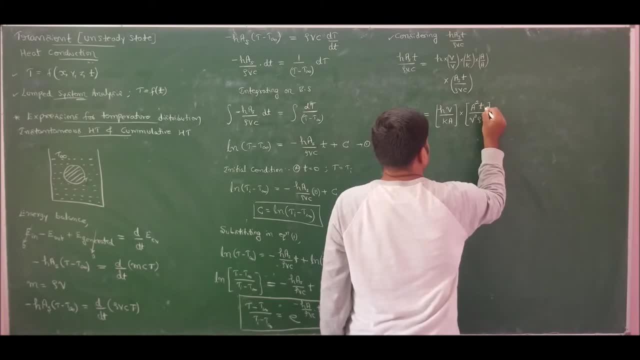 so I left out with K in a numerator. so now the ratio of volume by area is nothing but characteristic length LC by K into here I can write it as K by Rosie is thermal diffusivity. this you people already know. it is alpha T divided by. 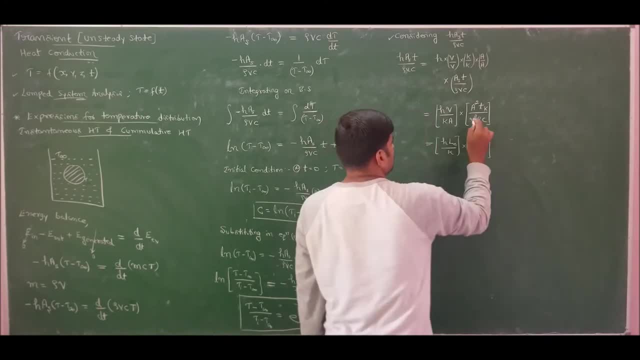 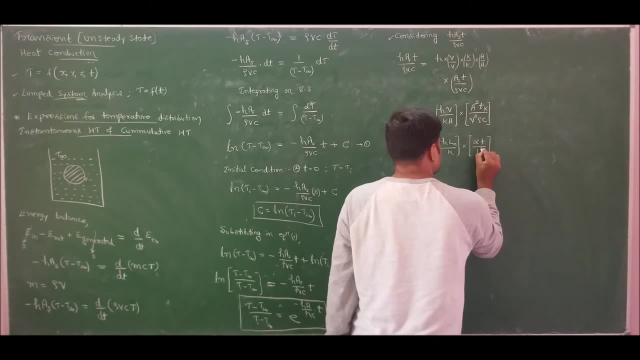 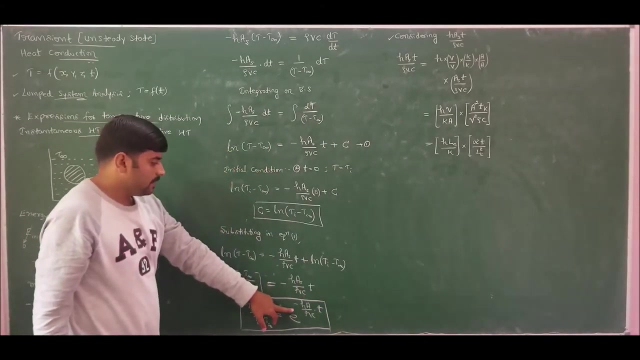 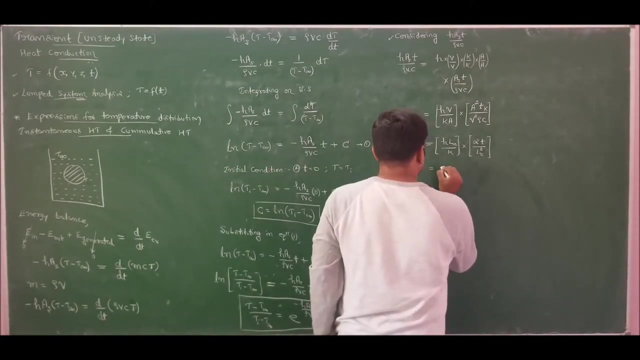 since we are volume square, become LC square. so this is what we get if I rearrange the term in the exponential ha by row. VCT can be rearranged like this. so why I rearranged like this is because of the reason this term is nothing but by art number. just now I have explained is: 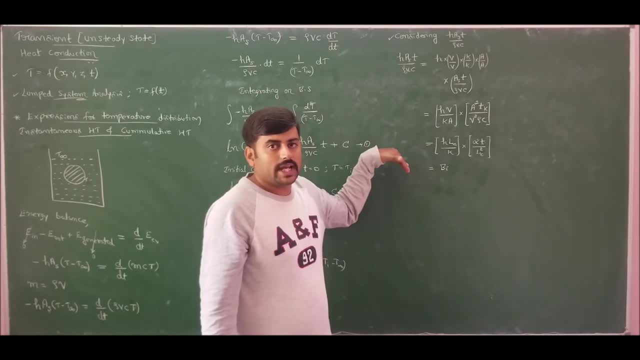 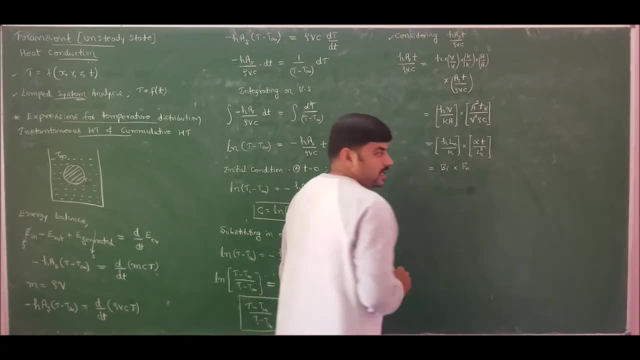 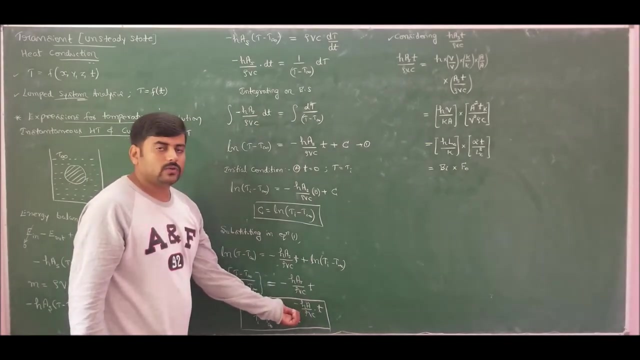 nothing but the ratio of of internal conductive resistance to external convective resistance times. the second term is called Fourier number, which is denoted by F4. So therefore the exponential can be written as e to the power of minus Biot number into. 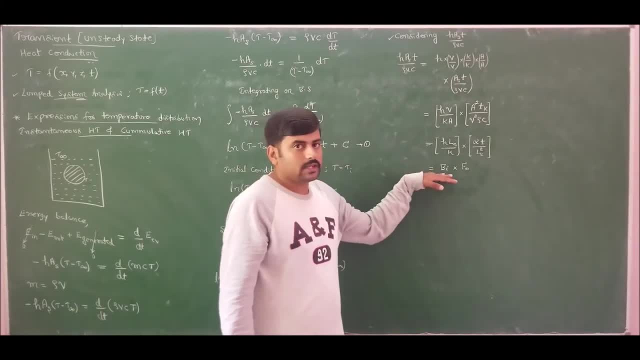 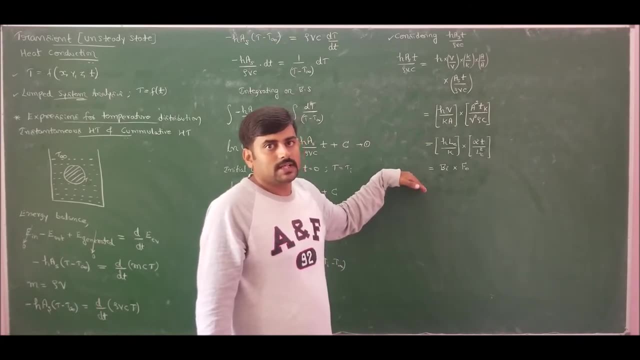 Fourier number. So the significance of Biot number is that if Biot number is less than 0.1, I can use Lumpur system analysis. that is, temperature is function of time alone. it is independent of space and also the internal conductive resistance is very small compared to external. 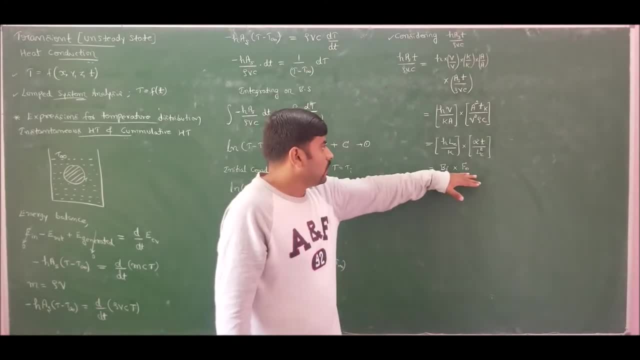 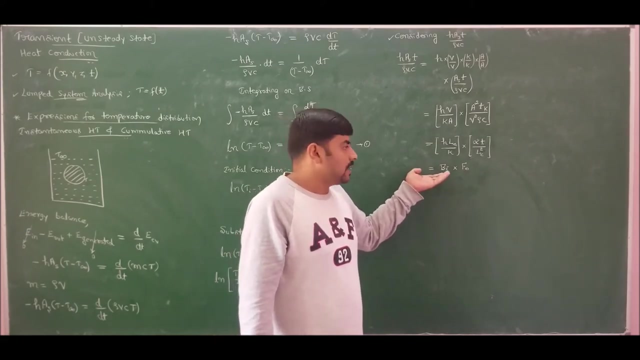 conductive, convective resistance, whereas Fourier number stands for the time duration, to the time required for heat to diffuse. So alpha stands for thermal diffusivity, which gives us how fast heat can penetrate inside the system. So this speaks about the time, and this is useful in determining the whether Lumpur. 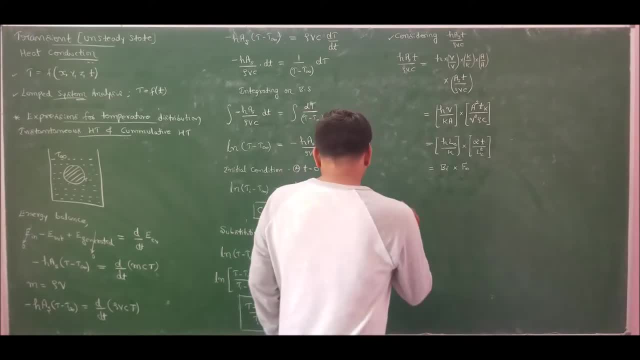 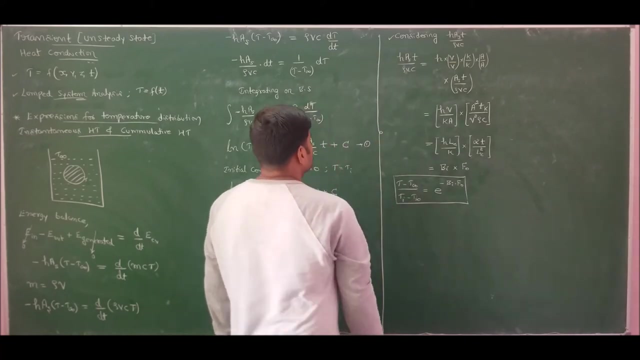 system analysis. Lumpur system analysis can be applied or not. So therefore I can write the temperature distribution as T minus T infinity by T. i minus T infinity is equal to e, to the power of minus Biot number into Fourier number Where, as I said, Lc. Lc is the characteristic length or geometric factor. 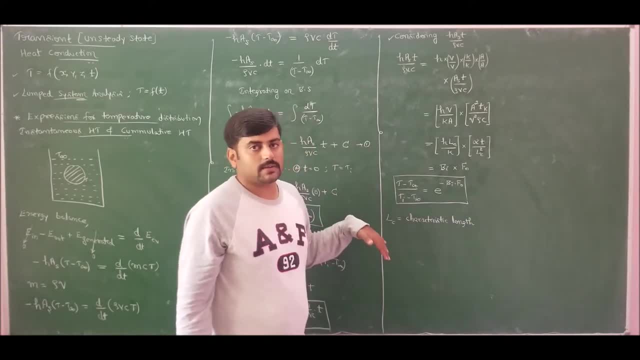 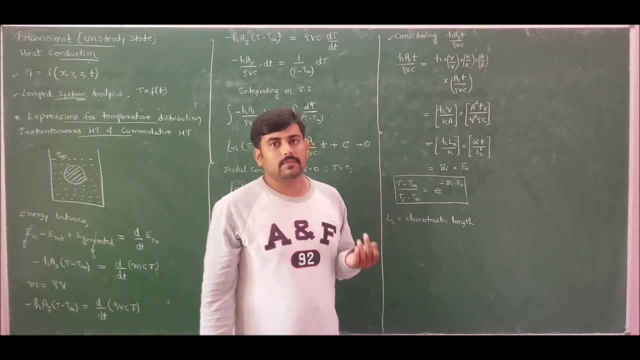 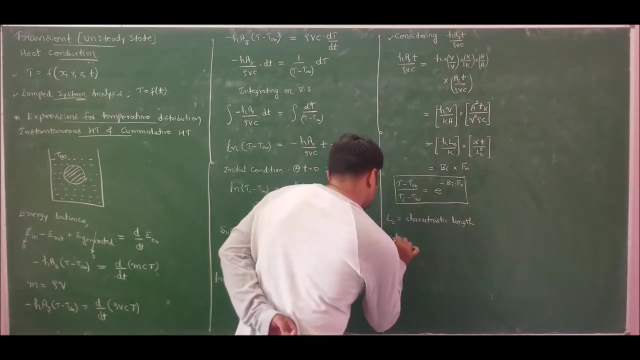 Characteristic length or geometric factor. So characteristic length is defined as the length over which the change in the temperature is desirable or which is observed. So characteristic length is the length over which the change in temperature is desirable for us. So the characteristic length for cylinders if I consider, if I consider a cylinder, 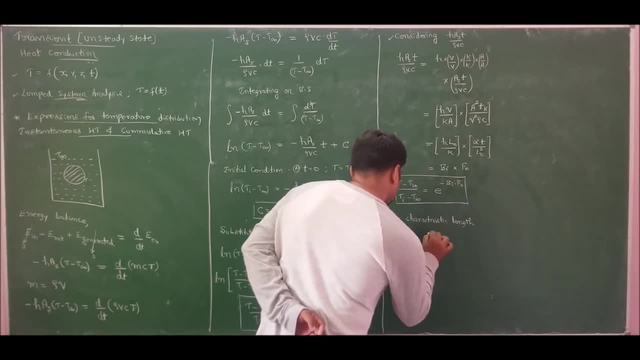 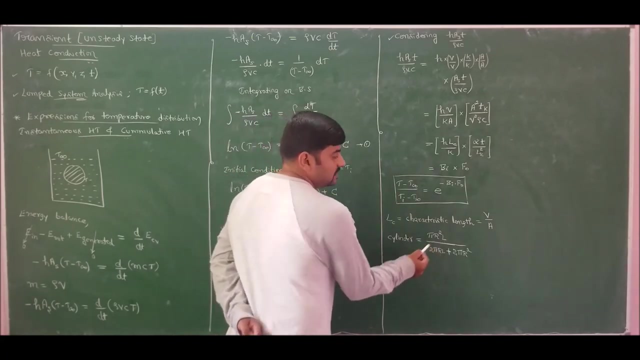 then characteristic length can be written as volume. Volume is y r squared L. Volume is L. Volume is L by surface area is 2 pi r n plus we have area at two end surfaces that is 2 pi r squared. If for a very long cylinder, if L is very large when compared to radius, then we can: 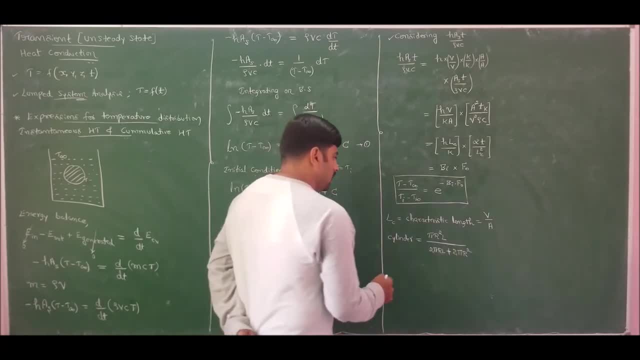 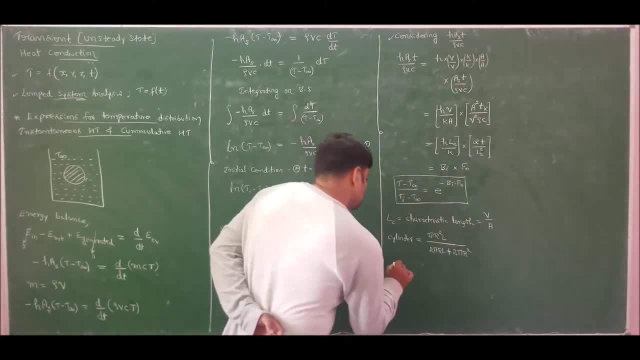 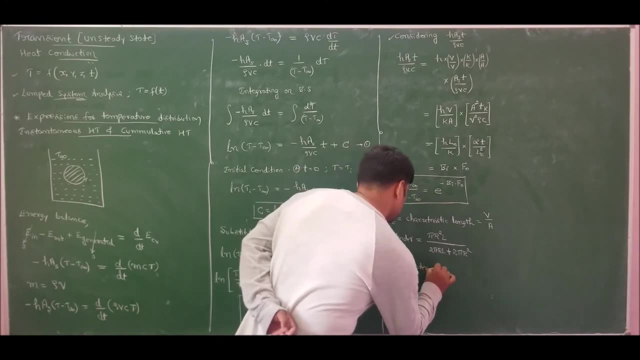 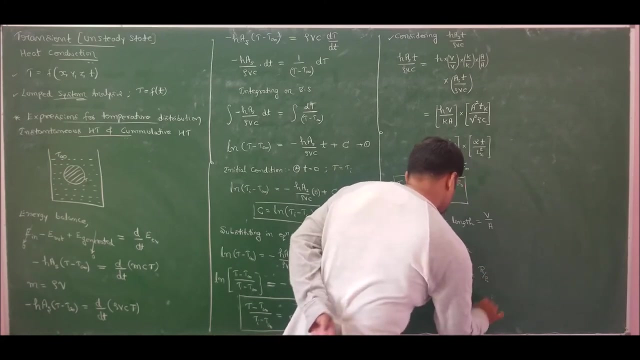 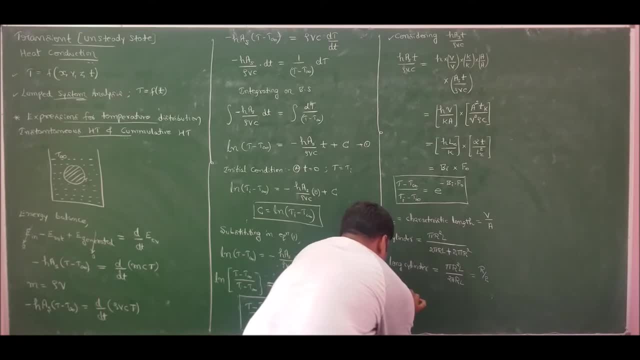 So for plates. for plates, if we consider we have volume as length into breadth, into thickness. let's take the thickness, as h divided by area is two, two times length into breadth, so therefore it is h by h stands for thickness, so which is nothing but semi thickness. 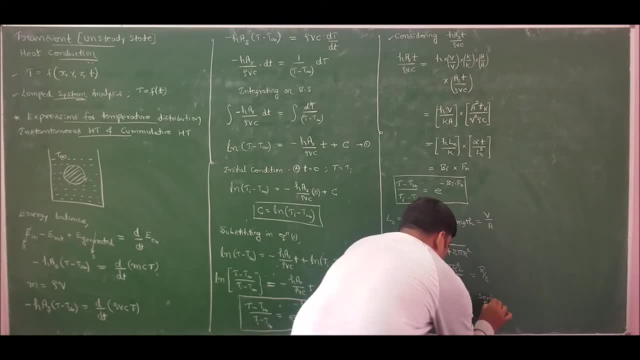 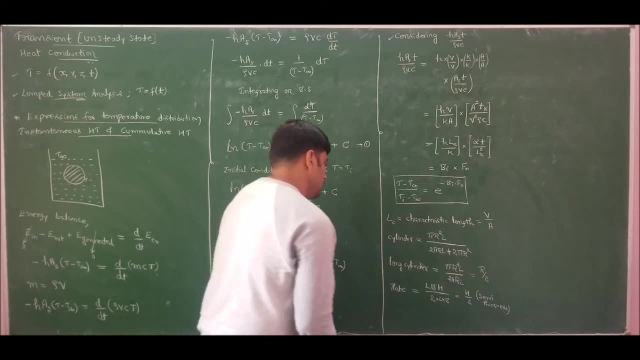 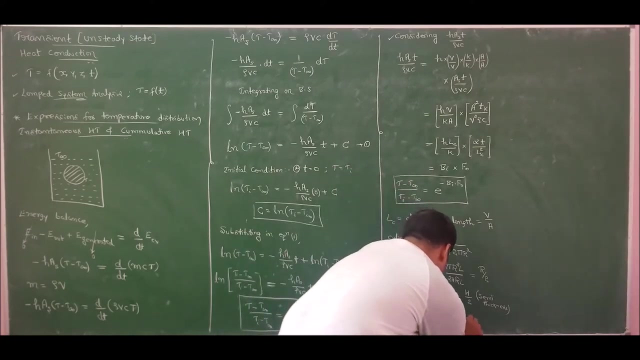 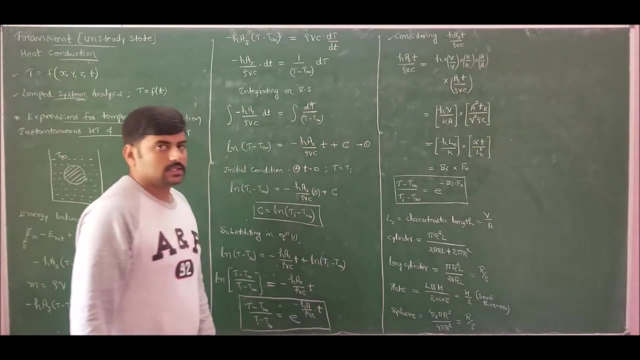 semi thickness. so similarly, if i consider for sphere, if i consider for sphere, y volume is 4 by 3 pi r cubed area is 4 pi r squared. so therefore characteristic length will become r by 3. so like this we can find the characteristic length. 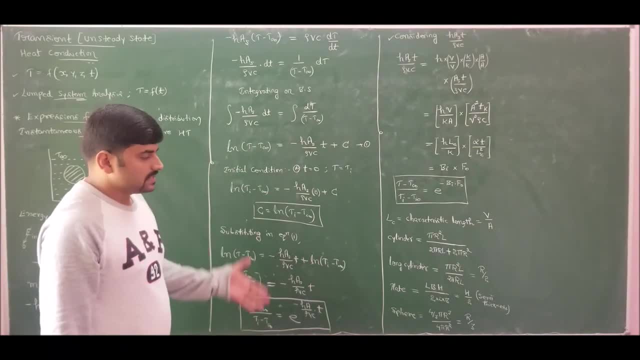 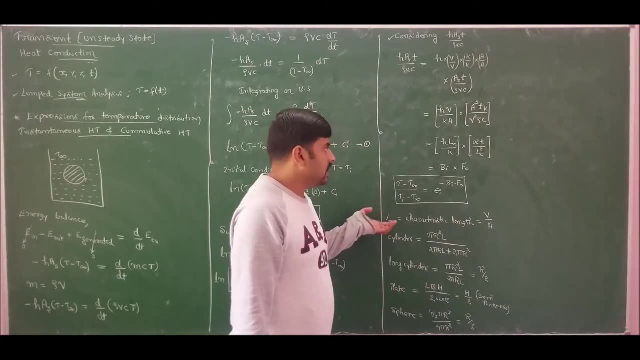 why this characteristic length is very, very important? because it is the length over which temperature change is desirable for us, and also, using this characteristic length, we are achieving the characteristics of the sphere. so this is called characteristic length. for this we have, in this way, length. only you can determine the biot number. biot number gives us whether the 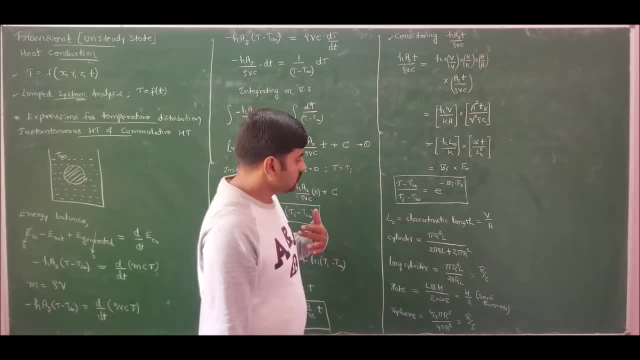 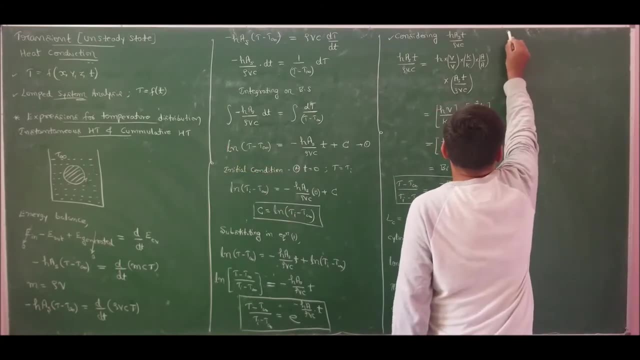 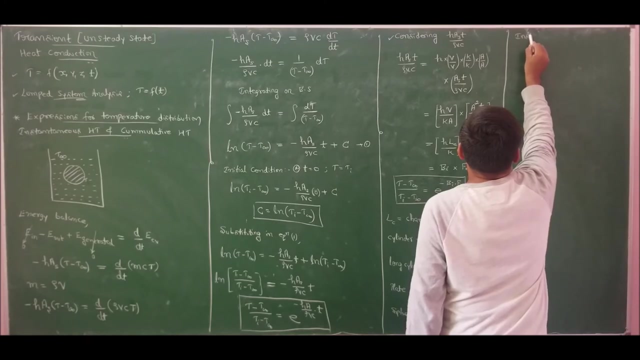 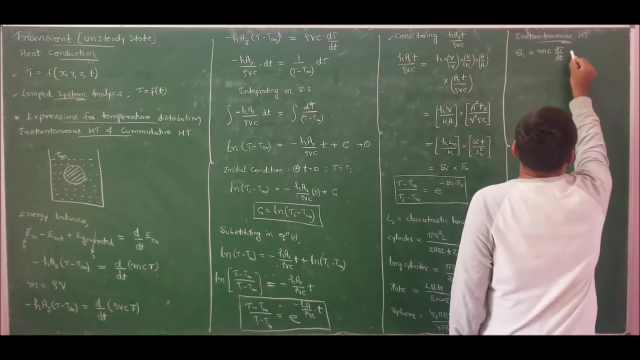 lumped system analysis can be employed or not. now moving ahead for calculation of instantaneous heat transfer. I mean for instantaneous heat transfer that is Q. instantaneous is equal to Mc. B became like, which is nothing but changing. internal energy of the system is equal to density transferred in the initial velocity of the voy kimchi liquid. we are not having an external energy of the system which is equal to density. 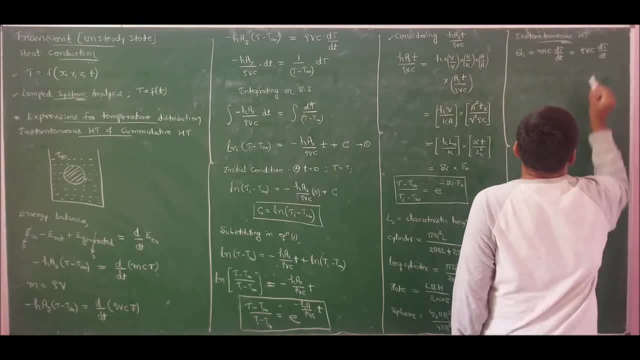 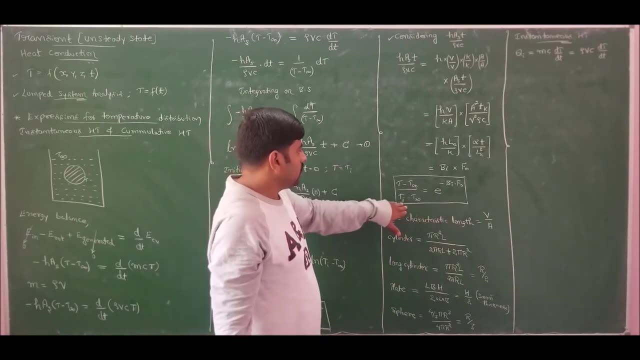 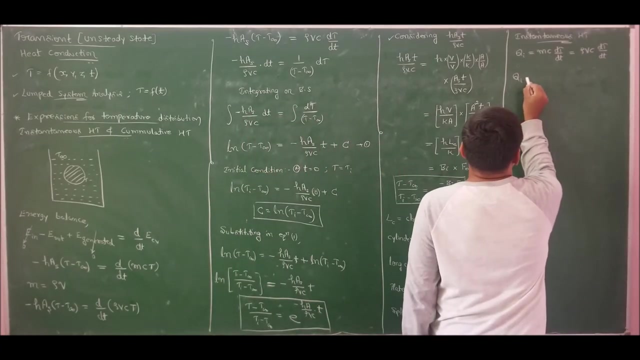 times volume into C, dT by dT. So we know the temperature distribution. So T is equal to e, to the power of Biot number into Fourier number, into Ti minus T infinity plus T infinity. So therefore, if I solve for instantaneous heat transfer, I will get rho BC d by dT of 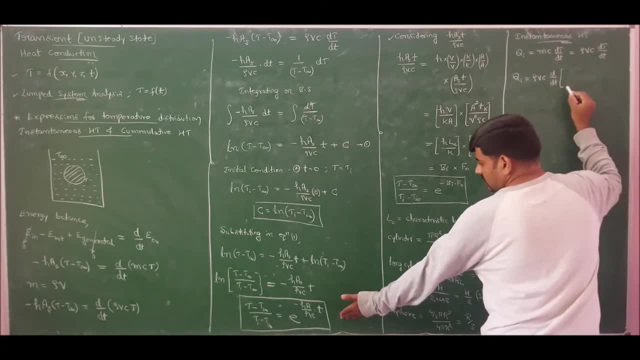 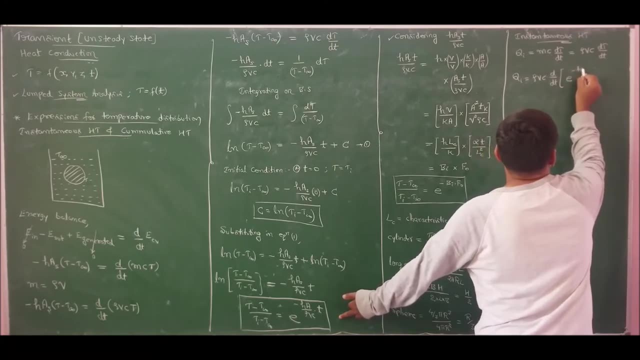 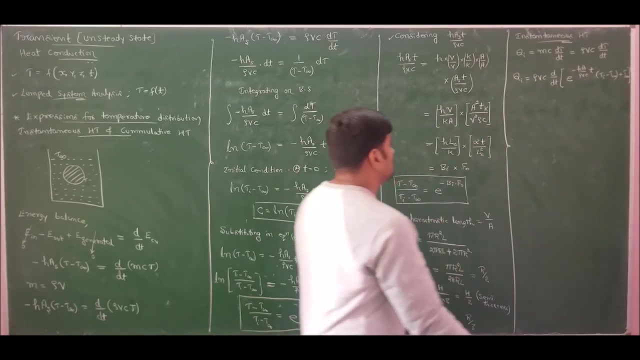 the value of T from this equation can be written as: T is equal to e, to the power of minus H, A by rho BC times time, into Ti minus T infinity, plus T infinity. So I realized the term to find the value of temperature T. 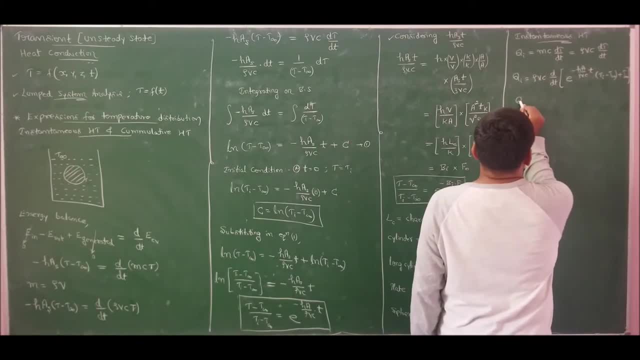 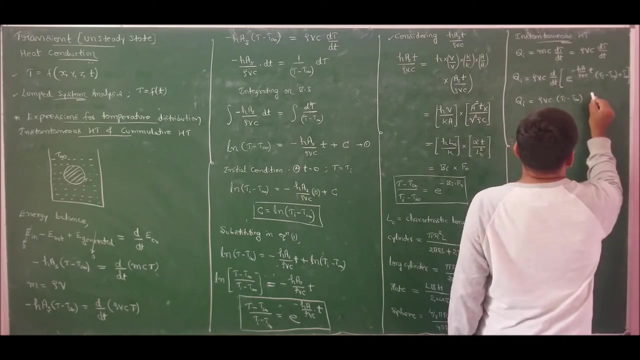 So now, if I differentiate and solve, I get the instantaneous heat transfer Qi as rho BC. So T, I minus T, infinity is constant. e to the power of Ax is A. e to the power of Ax minus H A by rho BC. e to the power of minus H A by rho BC T. So differentiate and solve. 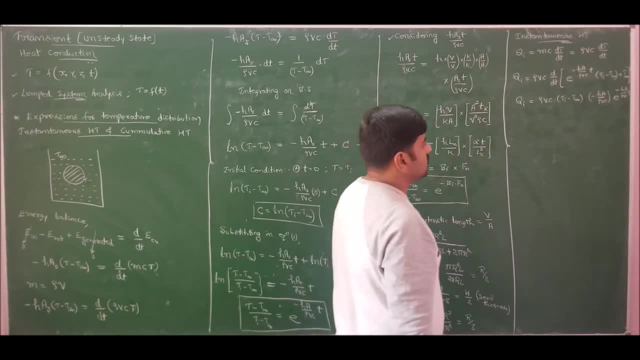 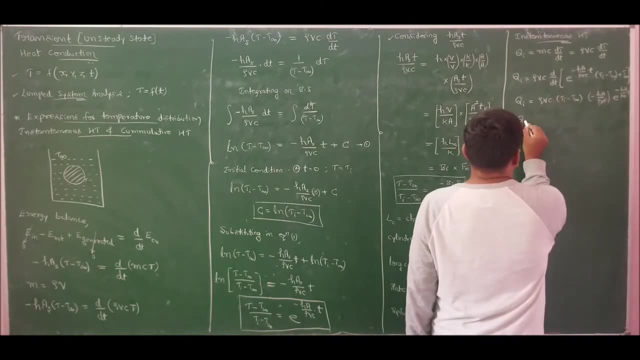 So if I differentiate and solve, I get the instantaneous heat transfer, Qi as rho BC times T. So if I want to celebrate the heat transfer, I can count on Q, I minus T and Q. I can say V, P, 2, e to the power, a to the power of half, raise to the power of 18 the power of a minus. 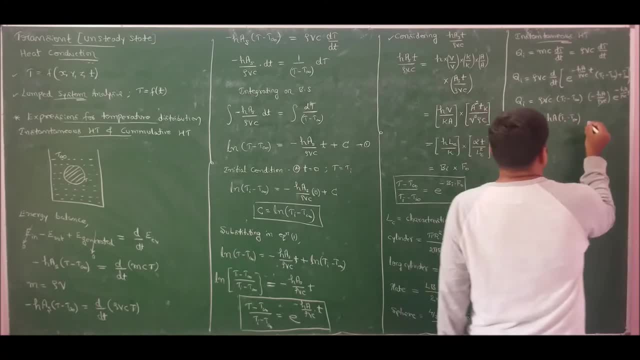 T A minus T, infinity b. So between three less than L s by Y is equal to minus H A times T. infinity is the duration of heat transfer. So if I rearrange the term, we can cancel out rho BC, rho VC, so therefore instantaneous. 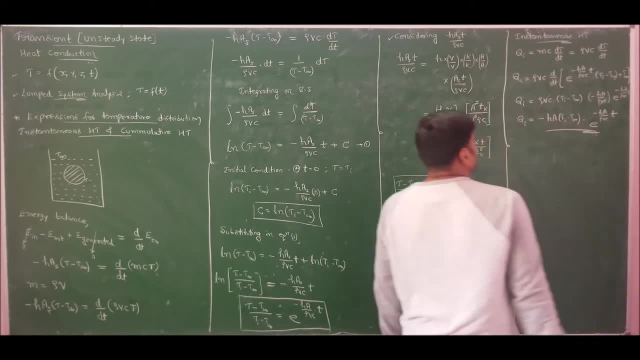 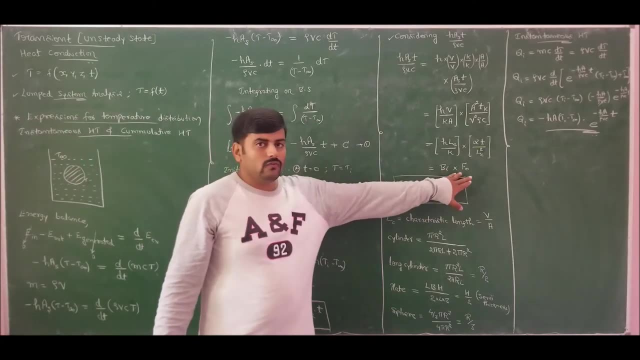 heat transfer Q I is equal to minus H, A, T, I, minus T, infinity into e, to the power of minus at A, x, rho BC times, b times. So this is the expression for instantaneous heat transfer. The value of HET by Rho BC can be written as Biot number into Fourier number. 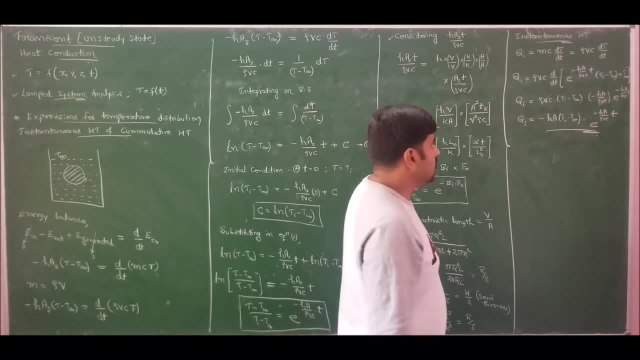 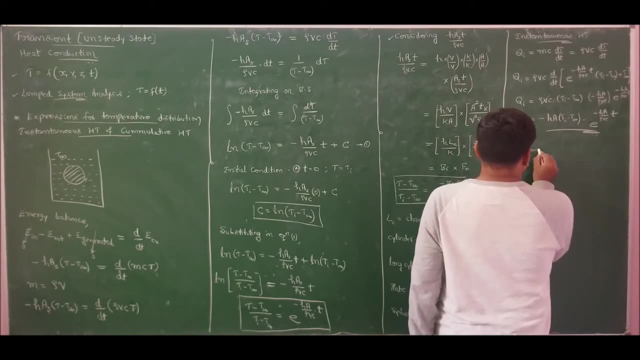 This you people already know. So this is the expression for instantaneous heat transfer. Next, moving for cumulative heat transfer. So cumulative heat transfer is given by integration over the time 0 to time t. the instantaneous heat transfer- So if I do I will get cumulative heat transfer as integral- is from 0 to t minus HA t, minus t, infinity b to the power of minus HA t by Rho BC dt. 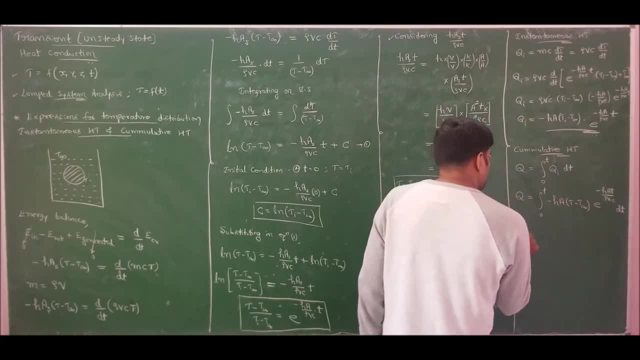 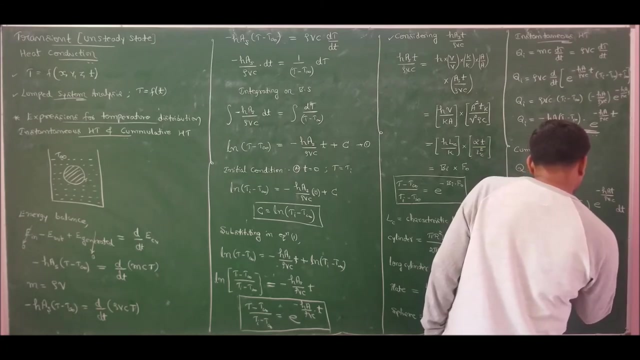 So now, if I perform integration, I will get the cumulative heat transfer Q as minus HA t minus t infinity. So integral of e power AX is e power AX by A, That is e to the power of minus HA, That is e to the power of minus HA t by Rho BC, divided by minus HA by Rho BC, whereas the limit varies from 0 to t. 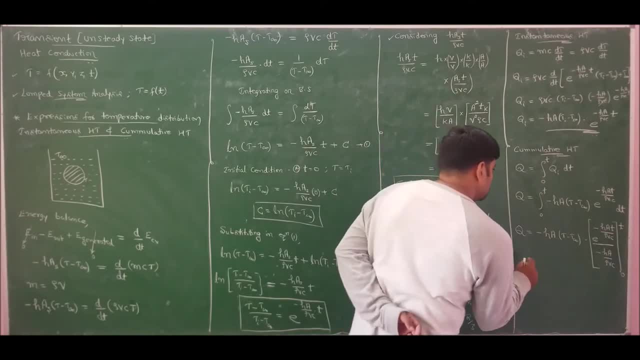 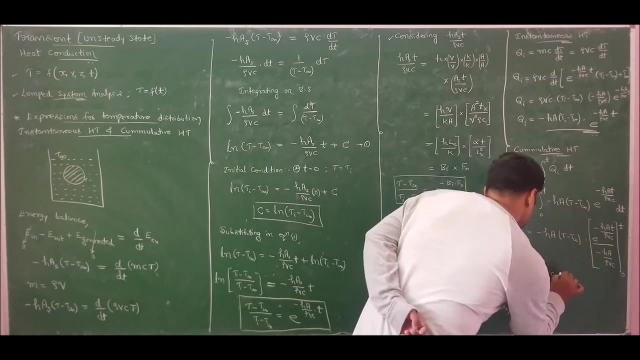 So if I simplify further, I will get cumulative heat transfer as minus of minus infinity. So if I simplify further, I will get cumulative heat transfer as minus of minus infinity, which become plus HA, and HA will get cancelled. I will get Rho BC t minus t infinity. 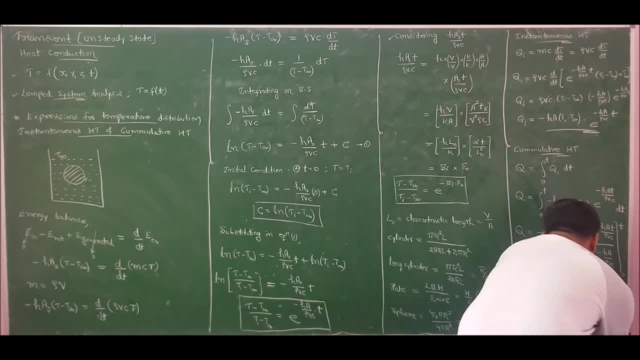 So, subtracting the limits, upper limit is t, That is, e to the power of minus HA, t by Rho, BC minus lower limit is 0, e to the power of 0 is 1.. So therefore The cumulative e-transfer is rho, vc t minus t, infinity times e to the power of minus. 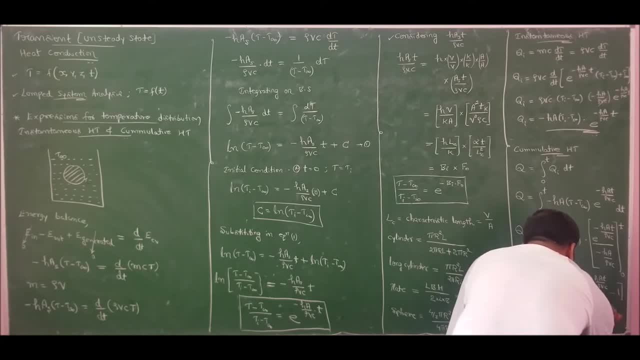 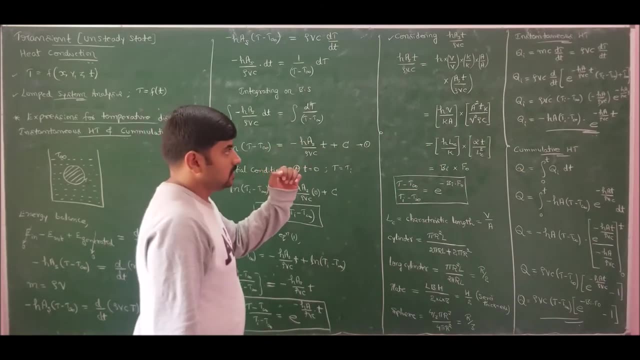 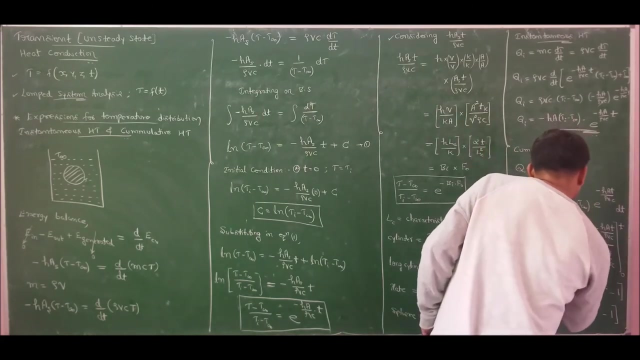 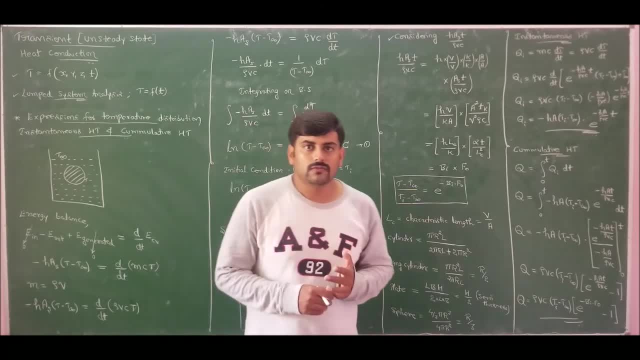 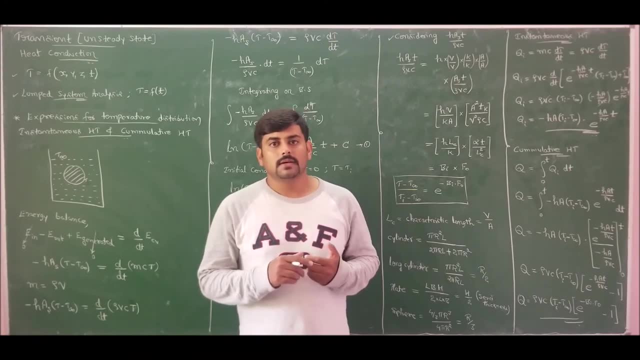 So so far, we have understood the meaning of transient e-transfer, the meaning of lumped system analysis, the meaning of characteristic length, the significance of Bayard number, significance of Fourier number and also expressions for characteristic length, and we have derived temperature distribution equation, instantaneous e-transfer and cumulative e-transfer equations. 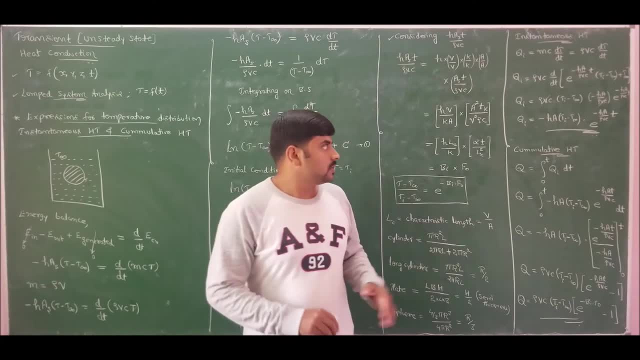 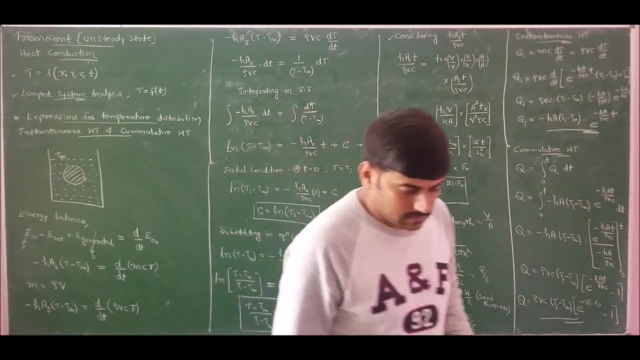 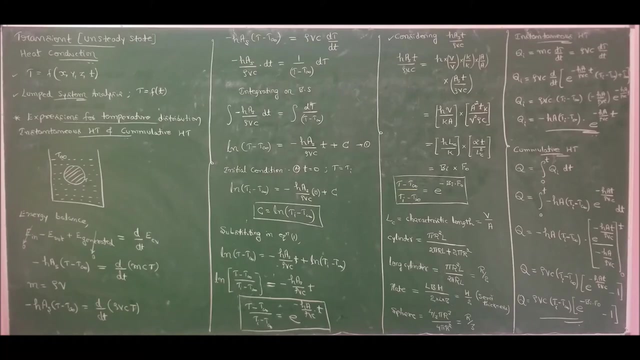 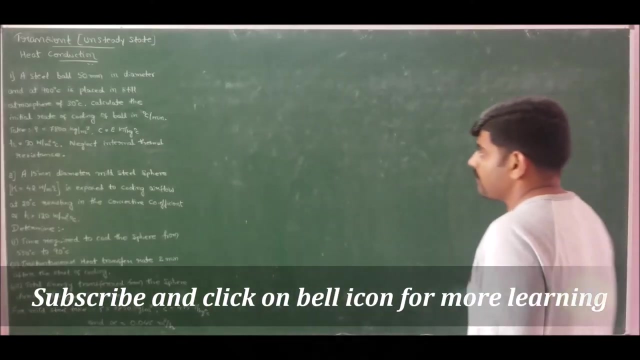 for one dimension transient heat conduction. So let me pause this video for a while so that people can copy it down Later. we will solve two numerical problems Now, moving ahead. the problem number one states that a steel ball 50 mm in diameter, 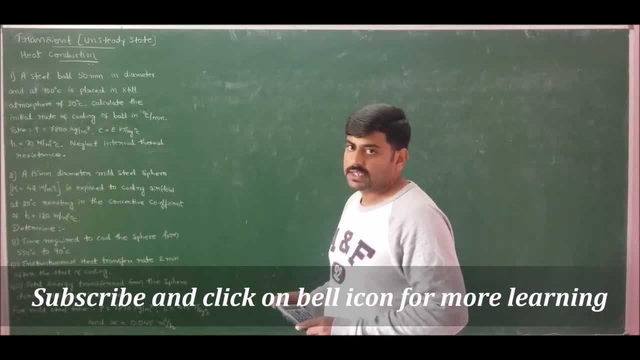 and at 900 degree Celsius, is placed in still atmosphere of 30 degree Celsius. Calculate the initial rate of cooling of ball in degree Celsius per minute. Take density as 0.5 bar per minute. Take density as 0.5 bar per minute. 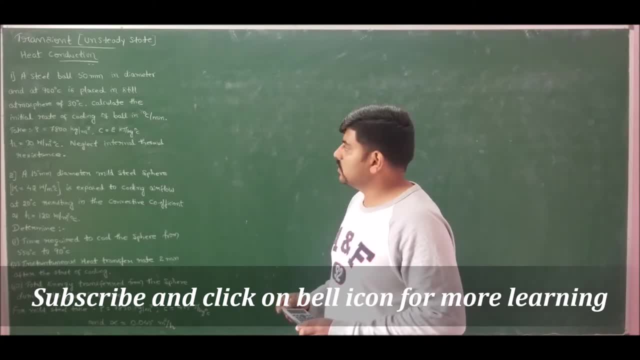 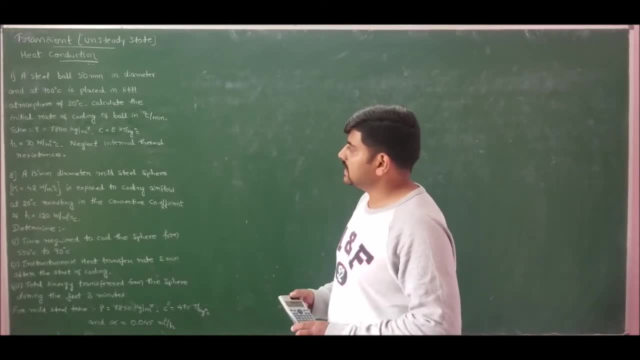 Goodbye. Take density as 7800 kg per meter cube, Specific heat as 2 kilojoules per kg degree Celsius, Thermect, unavreadable recruitment high 32 watt per meter KEP. Since heat himself is trading that net at indirect statement resistance we can use. 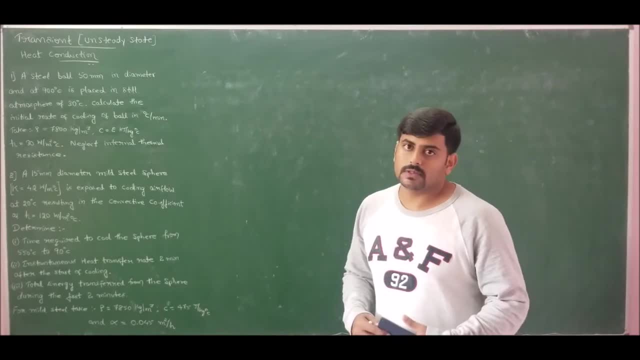 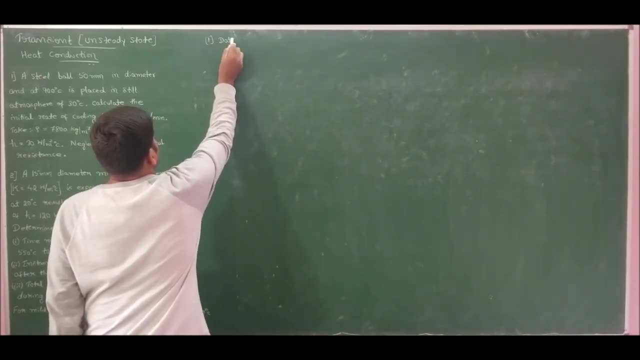 lumped theory to solve this problem. So if we restore the data given for bağ number one One, we have a steep ball of diameter AE1 in parcel. weight Unอง Dave II bar 1 GV' psycho queda dou Vary e Penceda extra gram M Neither com in. 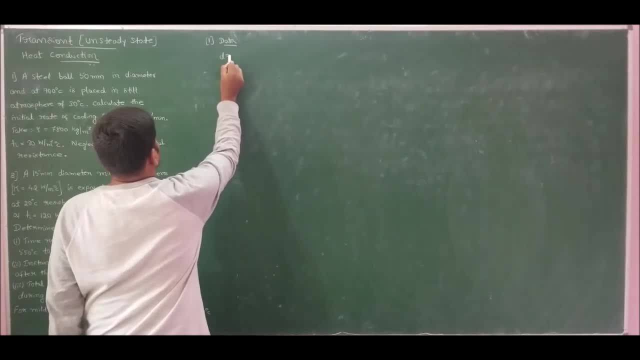 total number explained by in this match. So once again we're done. Earlier, 50 mm at 900 degree Celsius is. given the initial temperature as 900 degree Celsius, then atmosphere P infinity is 30 degree Celsius. calculate the rate of cooling of. 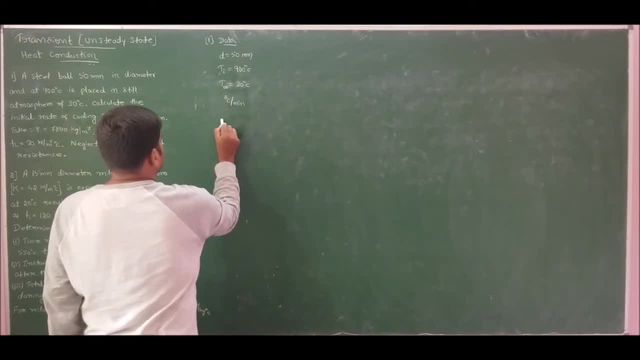 ball in degree Celsius per minute. so therefore time duration is given as one minute, so time is 60 seconds. take density as 7800 kg per meter cube and C as 2 kilojoules per kg degree Celsius and H as 30 watts per meter square degree Celsius. so since he is stating that neglect internal. 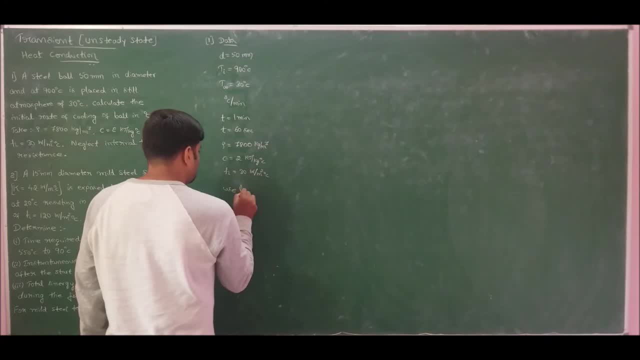 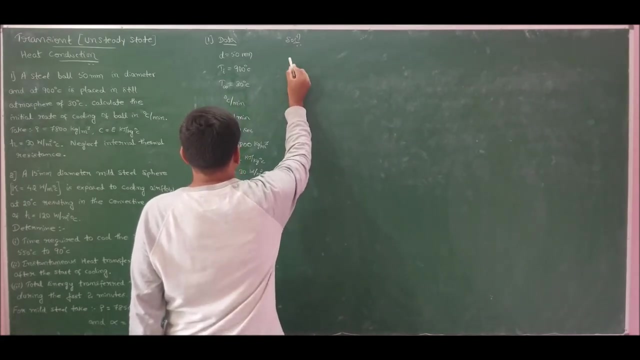 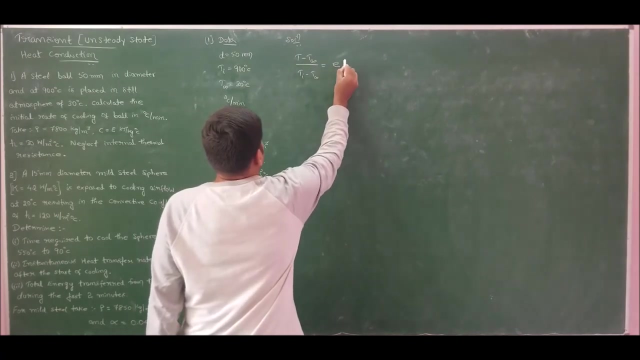 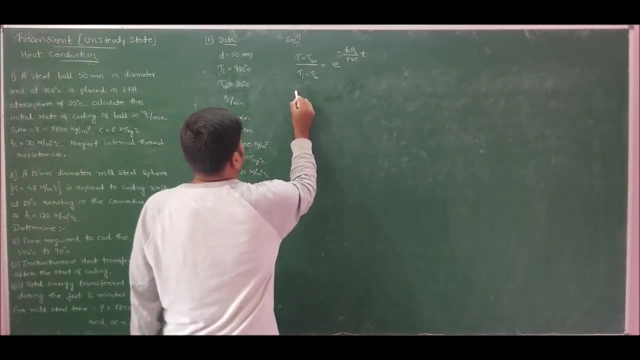 thermal resistance. we can use lump theory. so therefore, if I solve this problem, we have the formula for temperature distribution as T minus T infinity. by T minus T infinity is equal to e, to the power of minus HAS, by rho Vc T. now coming for Adulation of each values, we have surface area too. 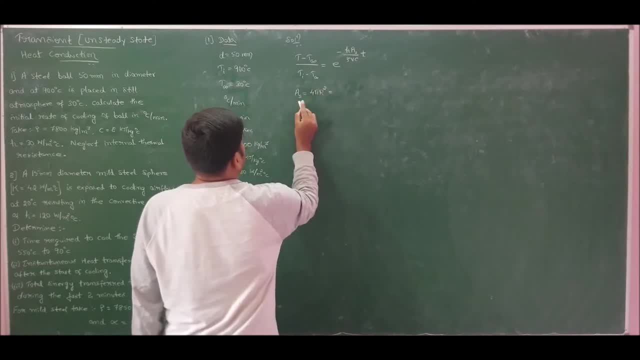 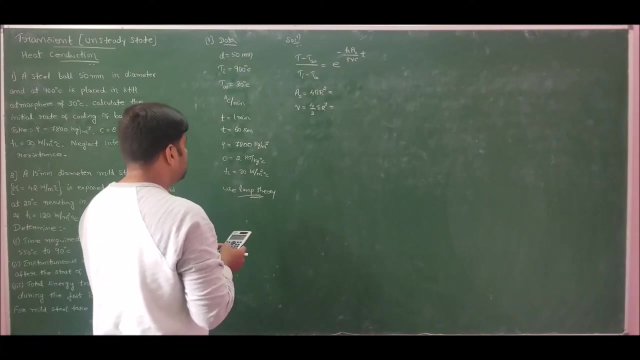 As 4.. square for sphere and volume is 4 by 3 pi r cube and we know all the values. so therefore, if I substitute and solve, I will get 4 into pi into. radius is 25 mm, that is 0.025 square. 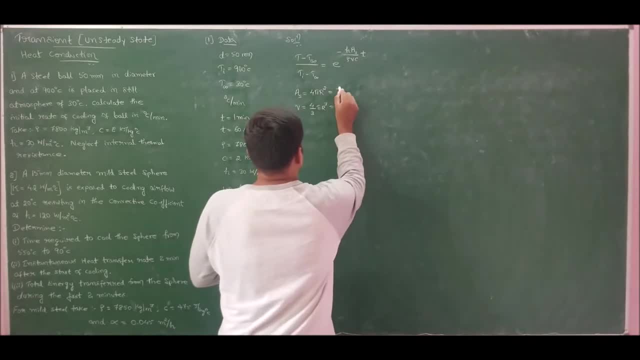 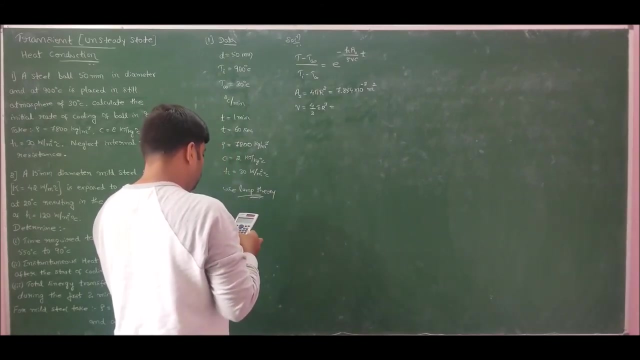 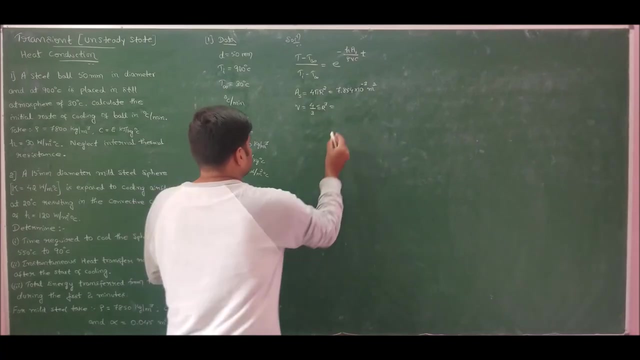 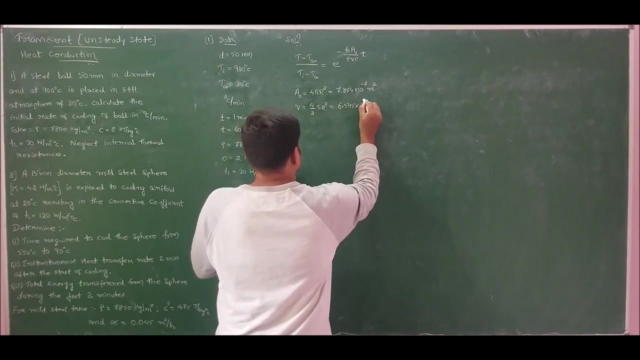 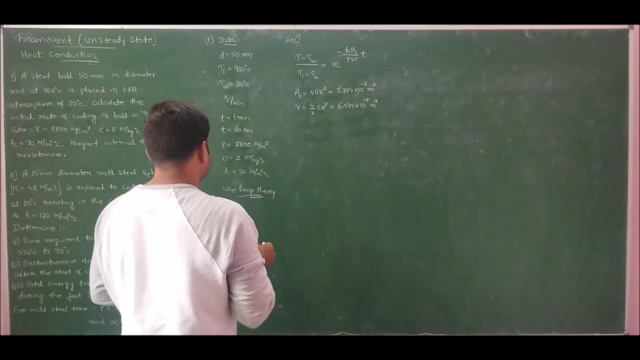 which is nothing but 7.854 into 20 to the power of minus 3 meter square. 4 by 3 pi r cube will be 6.545 into 10 to the power of minus 5 meter cube. so we know all the values. if I substitute: 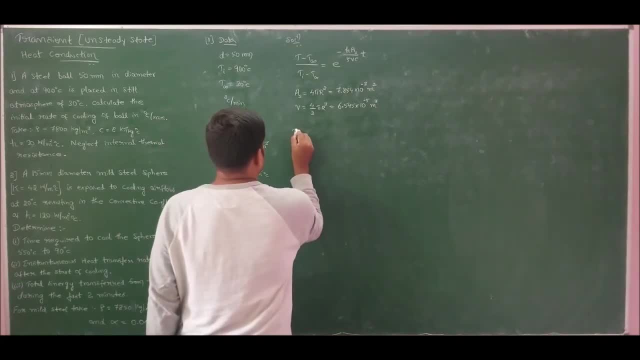 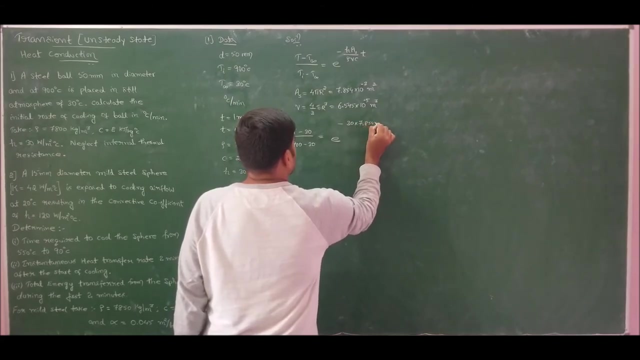 and solve. I will get the temperature as T minus T infinity is 30 degree Celsius. divided by initial temperature is 900 minus T infinity is 30 degree Celsius, which is equal to e, to the power of minus h is 30.. As we know, the temperature is 7.854 into 10 to the power of minus 3 into time is 60 seconds. 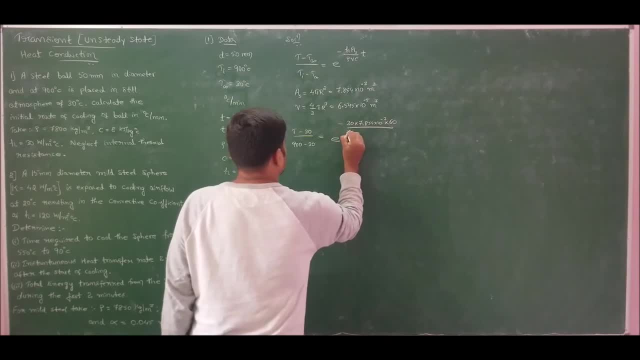 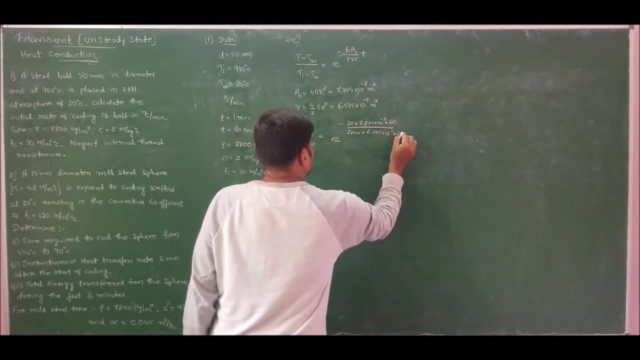 divided by density is 7800. into volume is 6.545 into 10. to the power of minus 5 into C is 2 kilo joules. so therefore it is 2 into 10 to the power of minus 3 into 10. to the. 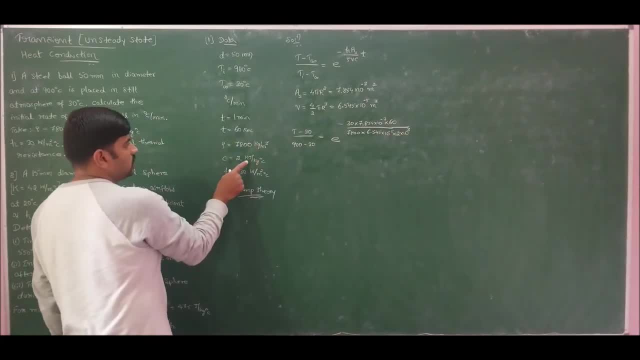 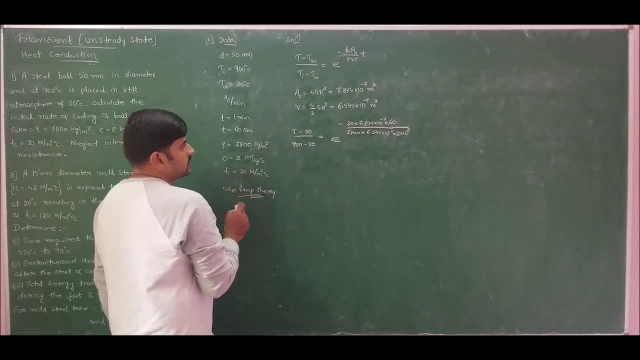 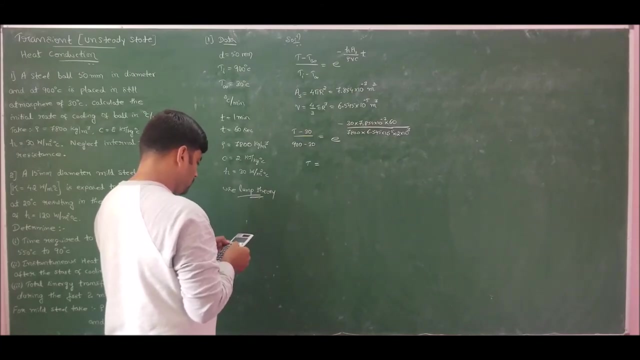 power of minus 6. so therefore it is 2 to the power of minus 7 into 10 to the power of minus 7. is very important: is given in kilo Joules per kg. it should be in joules per kg because h is in Wachts, is not in kilo wats. so maintain common units. so if we solve and 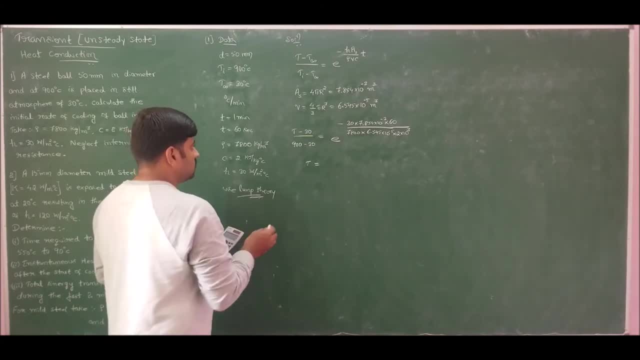 get the value of T as, which is equal to 0.986so therefore, T-30 by 0.986, and that is what we are getting at. so for joules per kg, quindi plus 5 joules per kg, that is the value of. 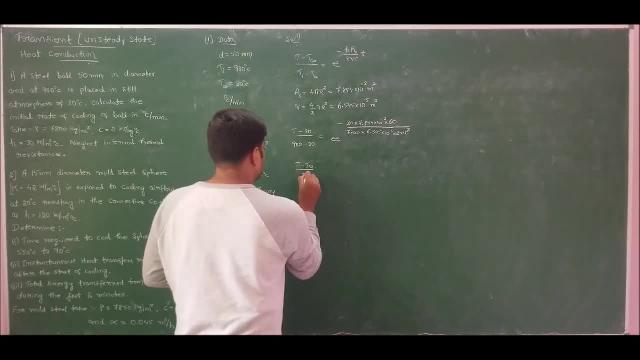 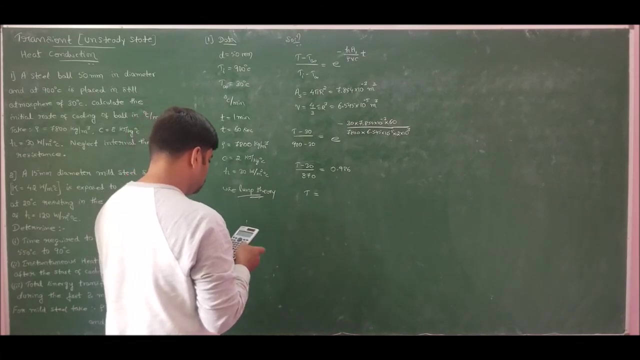 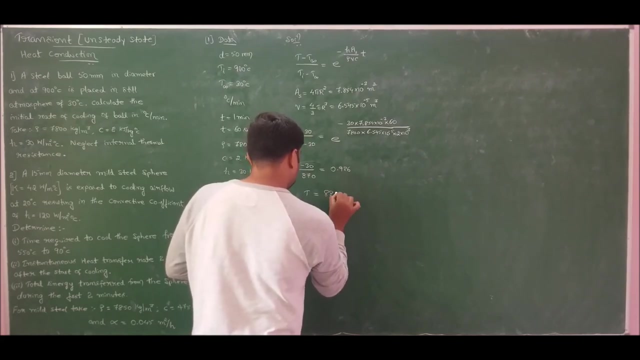 T and then for R to minus, a model as you can get value of Totted values. it is always n minus b of T, but we know this value as a integral and that is followed by til E, by to plus b. De도o 870 is equal to 0.986, so therefore T is equal to into 870 plus 30, which is equal to 888. I can take: 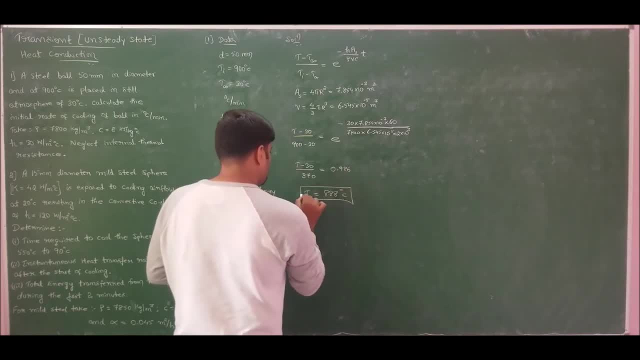 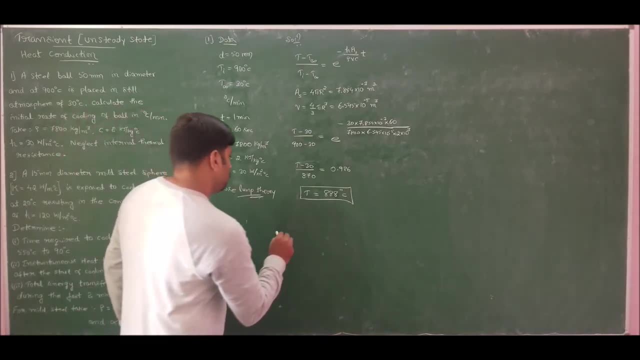 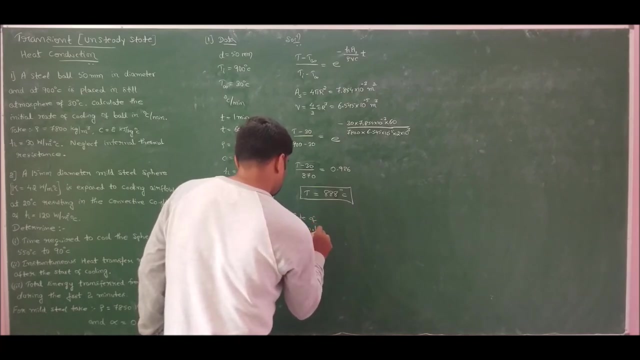 it as 888 degree Celsius, so this is the temperature after one minute, that is, after 60 seconds. so therefore rate of cooling will be: initially it is at 900 degree Celsius. after one minute it has become 888 degree Celsius, so the difference is 12 degree Celsius per one minute. so this: 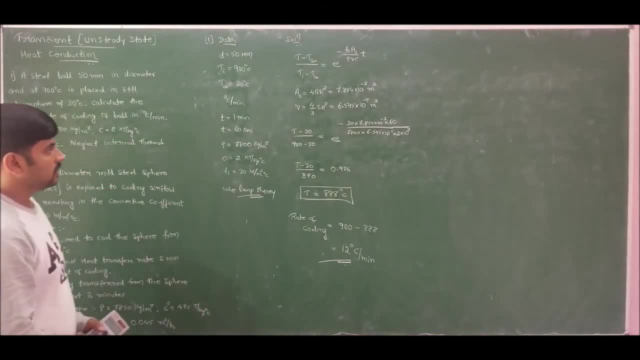 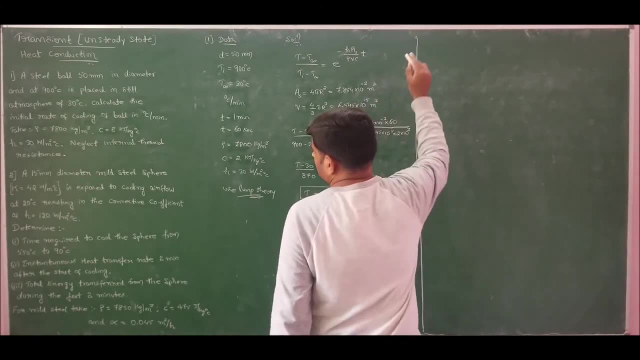 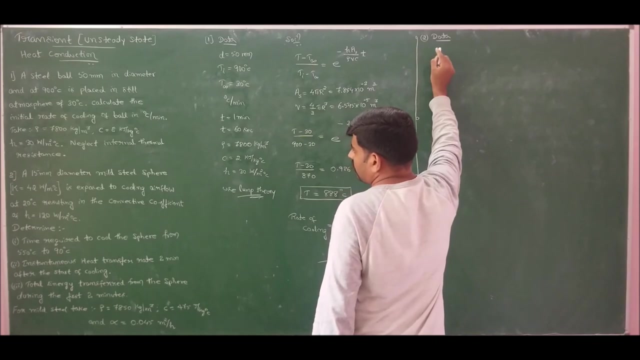 is the solution for problem number one. let us move for problem number two. moving for problem number two, the peristalti data given, we have a 15 mm diameter married steel sphere. we have given the diameter as 15 mm, with thermal conductivity K as 42 watt. 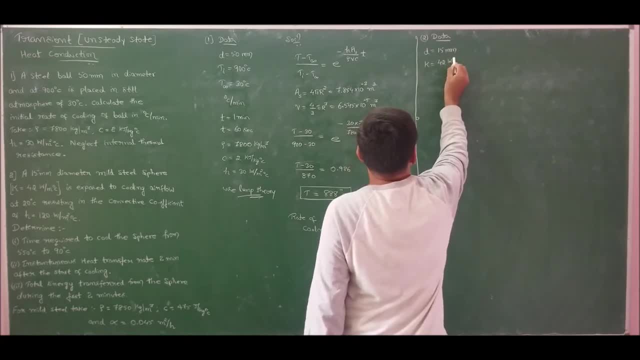 per meter degree Celsius, which is exposed to a cooling temperature which is equal to 880 degree Celsius. So this is the temperature. after one minute it has become 888 degree Celsius. so this is equal to 888 degree Celsius per minute. so we have given the moment, flow at T, infinity is 10 degree Celsius, resulting in convective. 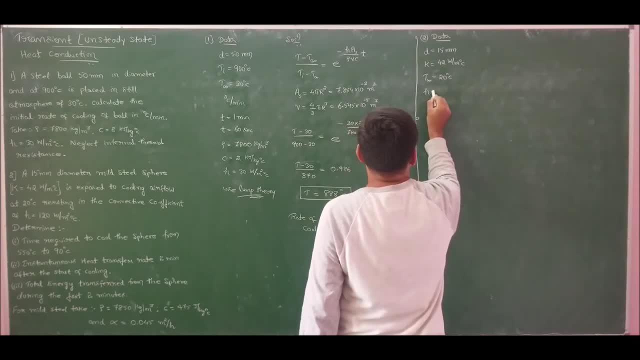 heat transfer coefficient of H: 120 watt per meter square degree Celsius. first one: determine time required for cooling the sphere from T i is 1100 watt per meter square degree Celsius. 550 degree Celsius to T of 90 degree Celsius. What is the time? Second one: Instantaneous. 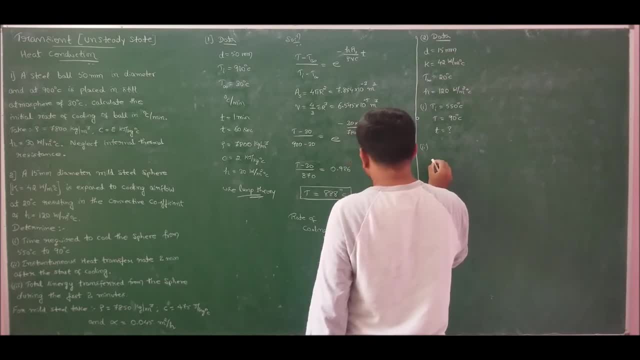 heat transfer rate 2 minutes after the start of cooling. So instantaneous heat transfer rate at 2 minutes. That is 2 into 60, which is equal to 120 seconds. And third one Total energy transfer from the sphere during the first 2 minutes. So total energy transfer. 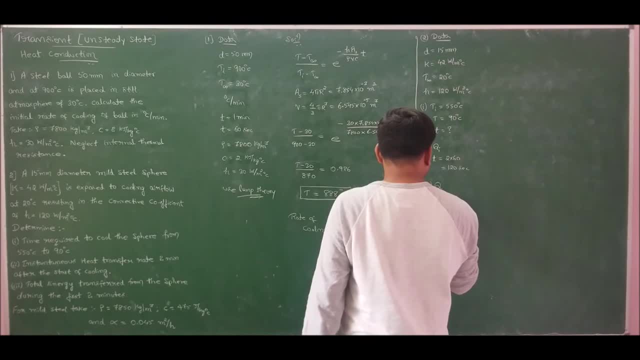 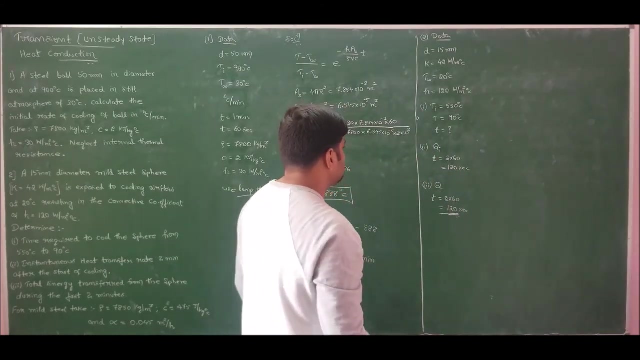 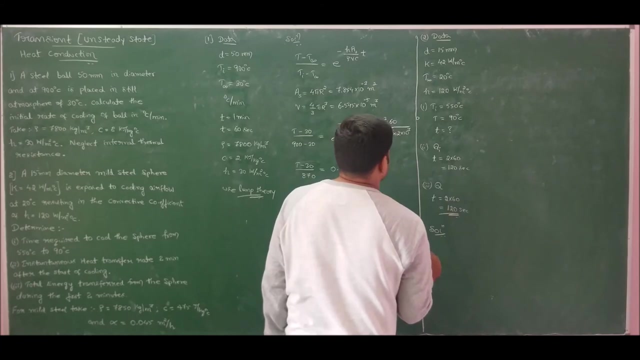 during first 2 minutes, That is, 2 into 60 seconds, which is equal to 120 seconds. So it is given the value of density, specific heat and thermal diffusivity for us Now. first let us verify whether lumped parameter analysis can be employed or not by using Biot number. 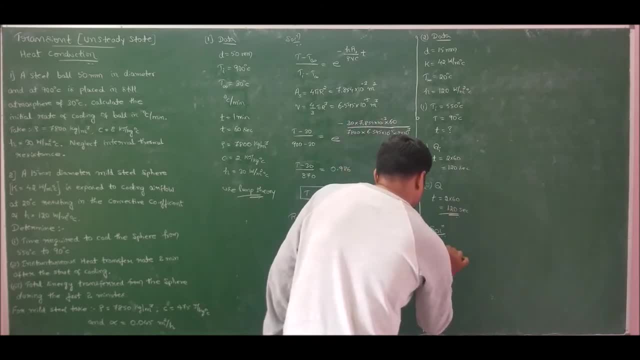 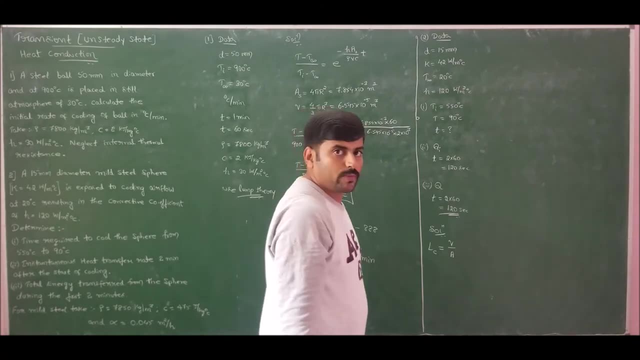 So for sphere we know that characteristic length LC is volume by area. where volume is 4 by 3 pi r, cube area is 4 pi r square. If we solve, I will get the formula as radius by 3 pi r. So I will get the formula as radius by 3 pi r. So I will get the formula as radius. 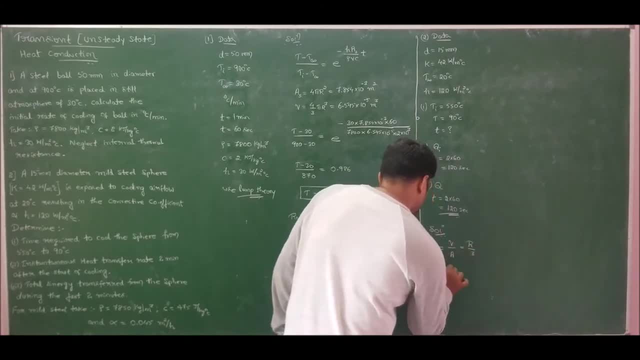 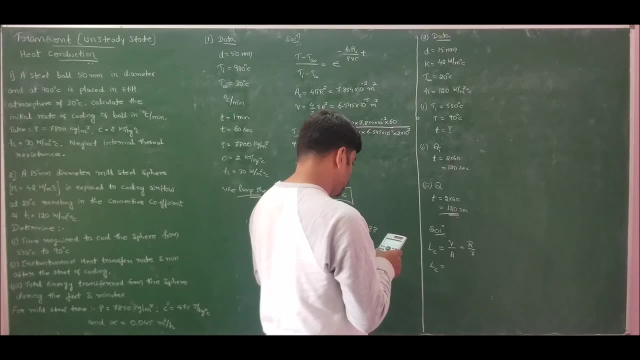 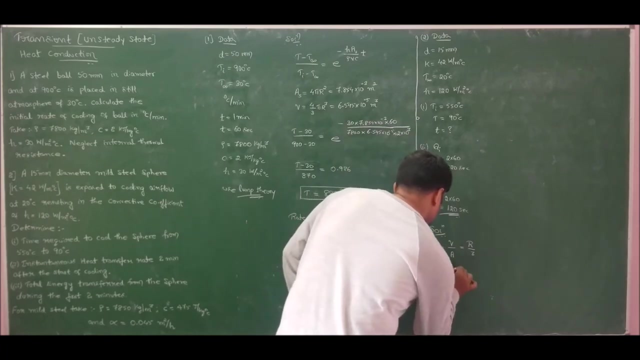 by 3 pi r. So therefore, characteristic length is 15, by 2 is 7.5, divided by 3, which is 2.5 mm, which is nothing but 0.0025 meters. So therefore, calculate the Biot number: Biot. 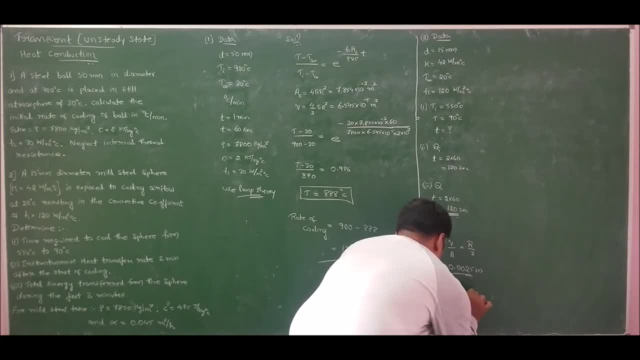 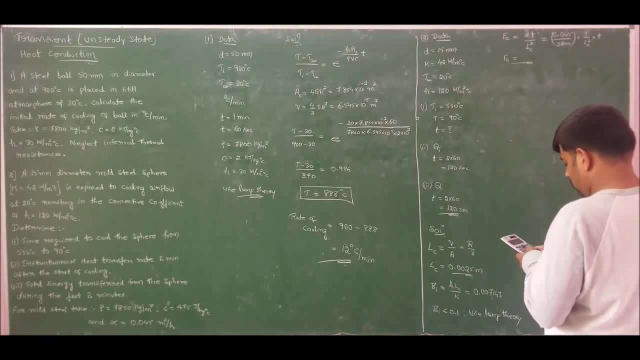 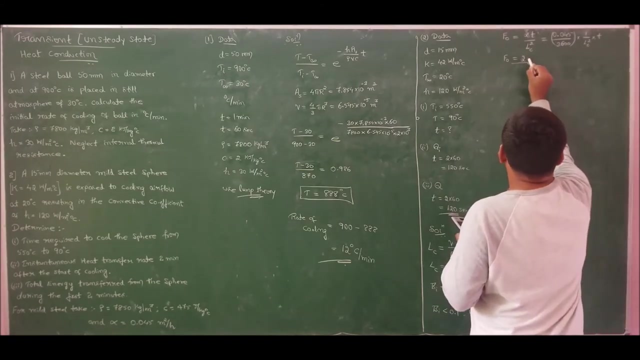 is 0.007143.. So since Biot number is 0.007143.. So since Biot number is 0.007143.. So since 600 into 1 by LC square, LC is 0.0025 square, you get the answer as 2t. so now first one. 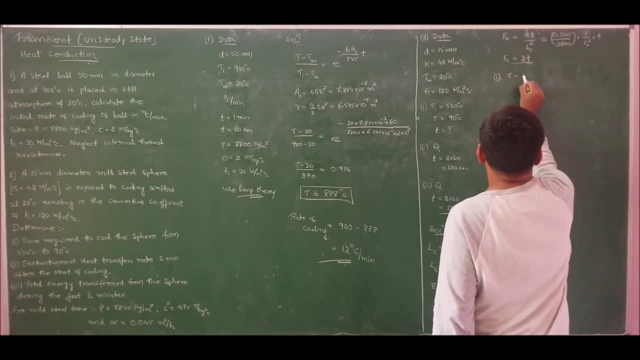 find the time. we said you know that temperature distribution is given by T minus T infinity, by TI minus T infinity is equal to e, to the power of minus by our number into Fourier number. so therefore you know all the values. if I substitute and solve, I will get 90 minus. 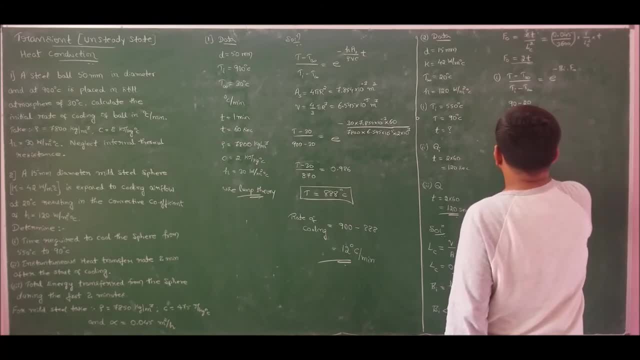 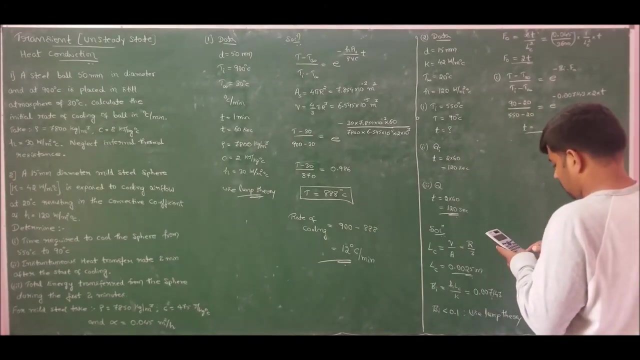 20 divided by T infinity, So T is equal to 550. minus 20 is equal to e, to the power of minus 0.007143 into Fourier number is 2t, so therefore T is equal to. in seconds I will get the answer, as T is equal. 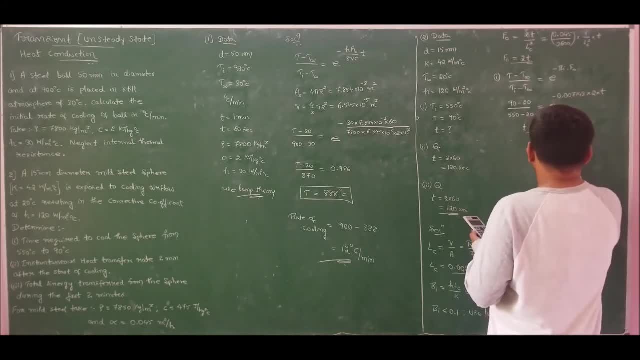 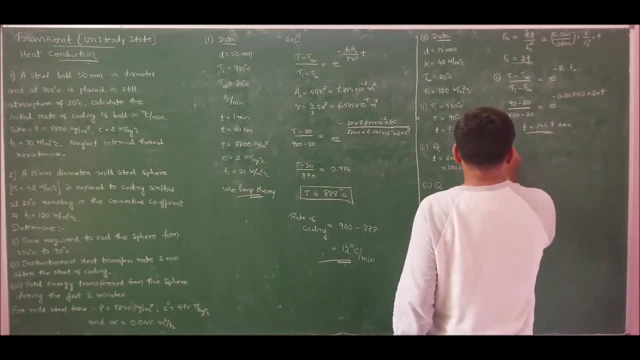 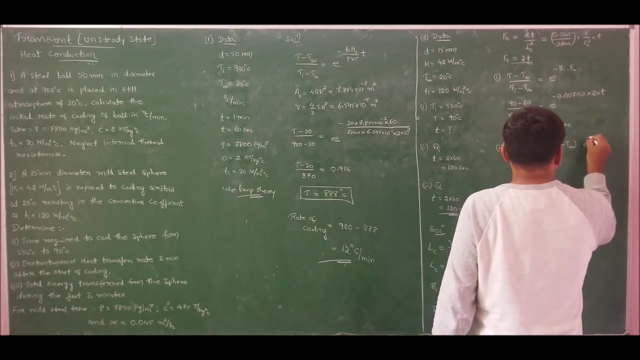 Next move for second one: instantaneous heat transfer. you know that instantaneous heat transfer is given by minus HAS, TI, minus T, infinity e, to the power of minus by our number into Fourier number. so therefore, instantaneous heat transfer is equal to minus H is 120 minus. 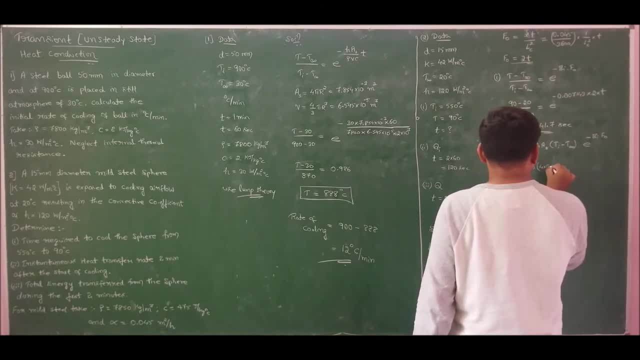 Area is 4 pi r square. Radius is 7.5 mm, That is 0.075.. 4 pi r square into T i T i is 550. into T, infinity is 20. into e, to the power of minus pi r number is 0.5.. 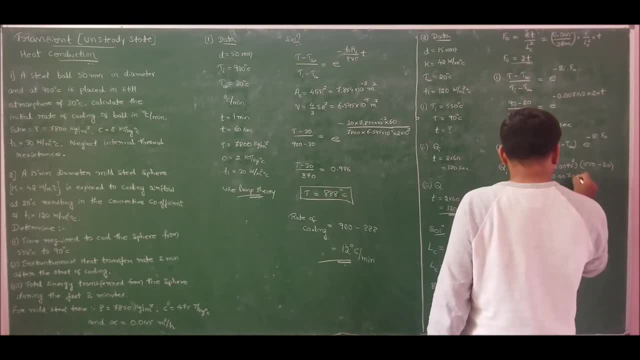 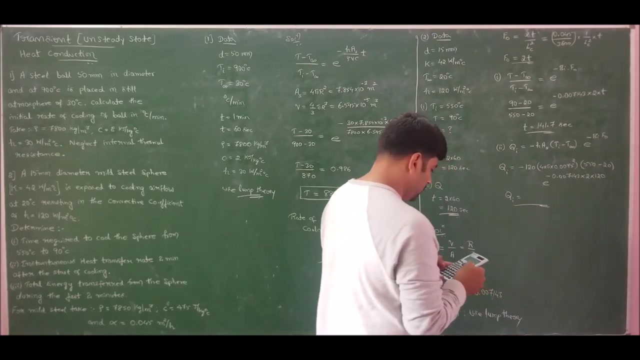 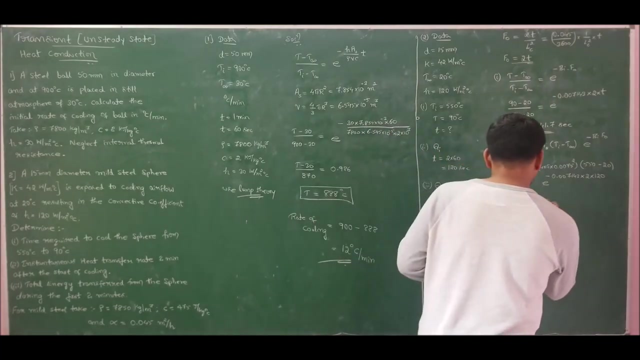 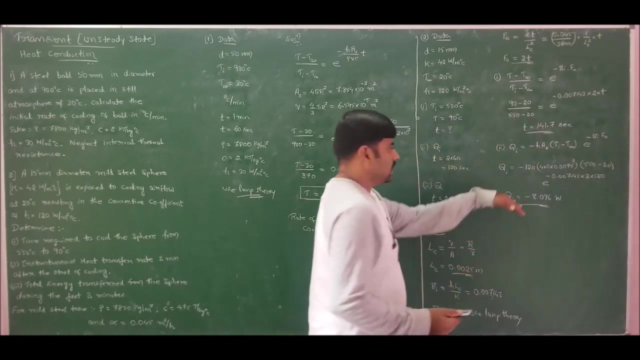 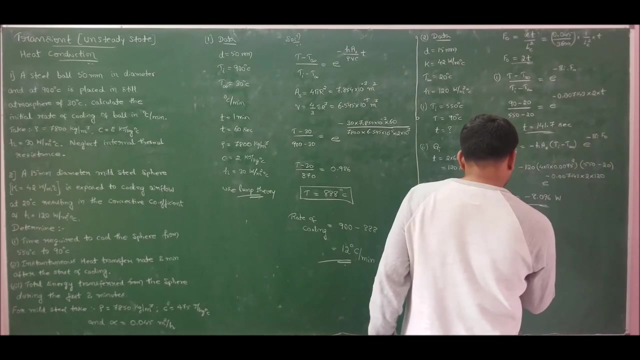 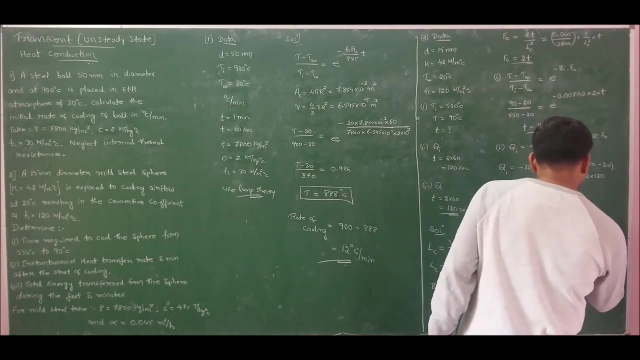 That is 0.07143, into 4 r number is 2 times T is 120 seconds. 2 T is 120 seconds. So therefore instantaneous heat transfer will be minus 8.096. Max. So here negative sign indicates that sphere is losing heat. Next move for third one Cumulative heat transfer which is given by rho vc T i minus T, infinity e to the power of minus pi r number into 4 r number minus 1.. 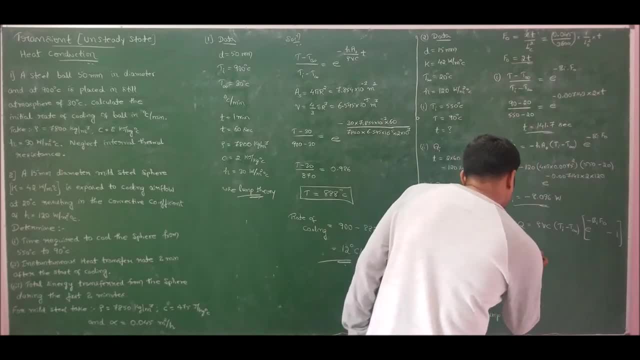 So this we have derived. So if I substitute and solve, I will get the answer as rho, vc, Rho is 7850.. V is 4 by 3 pi r cube, 0.0075 cube, into T. i is 550 into T, infinity is 20.. 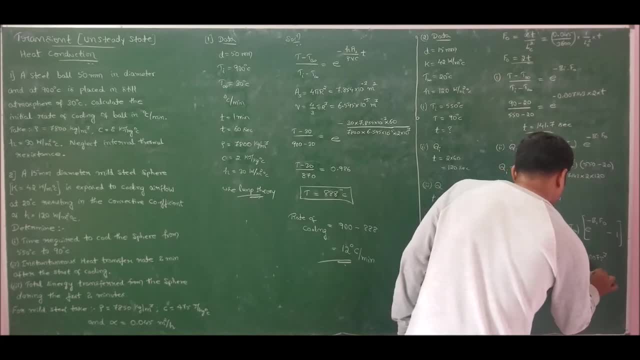 This same also. we will calculate this prime square into ear cube into e to the power of minus 4 pi r number, That is 0.10143 E U to the power of minus by 0 into 4 e r minus 1.. 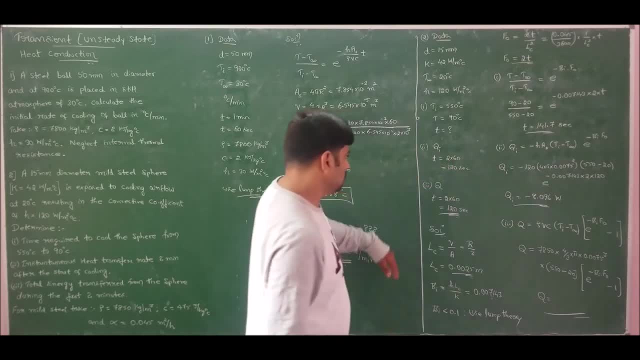 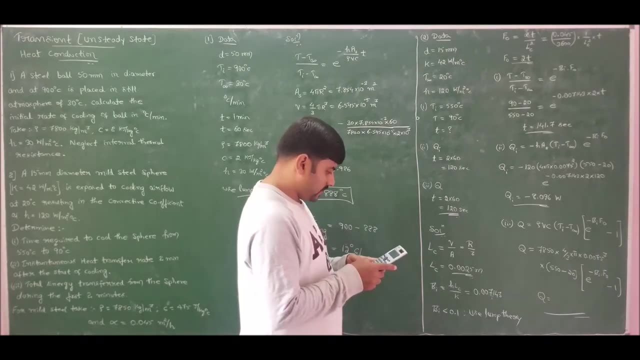 So if I solve I will get the answer as So in case of 4 e r number I will substitute T as 120 and solve: That is 7850 invt 4 by 3 pi times R, cube 0, moral double 075.. 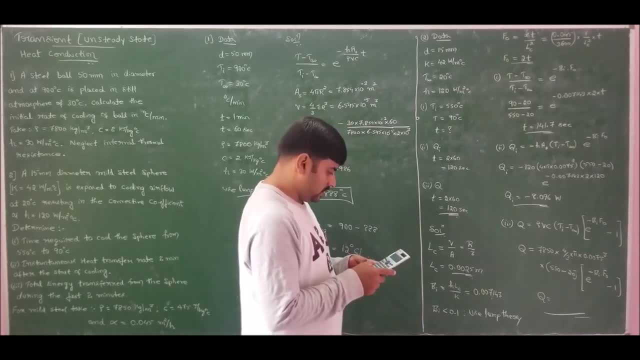 That is 7850roads into 4 y, 3 pi times R cube, 0 pol double 075 cube. into 3 pi times 0.00075 square. in PE times 0.00075 square There is a good totalく into 550 minus 20, into e to the power of minus bio number is 0.007143. into 2 times t is 120 minus 1..